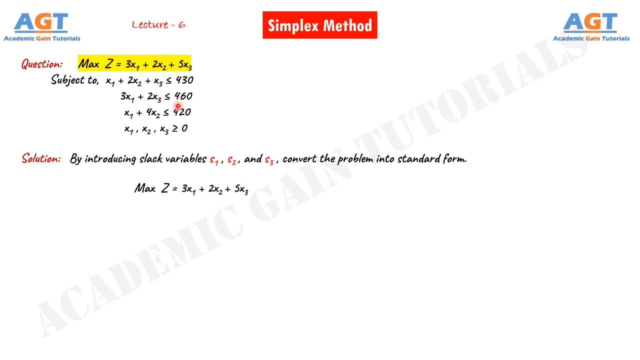 So the objective function here is: 3 times y is equal to 3 vector x1 plus 2, x2 plus 5 x3.. Now Let's write the constraints. Here we have the constraints as we can see here. 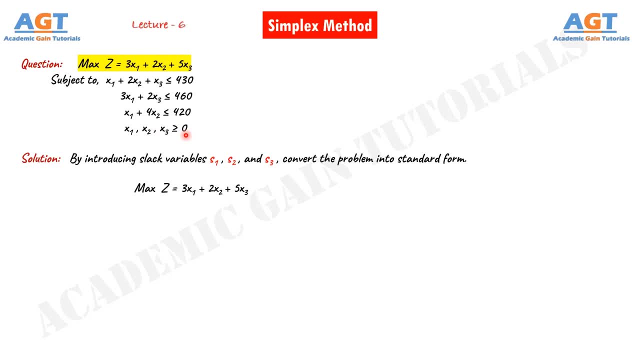 The decision variables x1,, x2, and x3 are all 0, So we don't have to change the decision variables in the constraints. If there were any unrestricted decision variables, then we would have to rewrite the constraint in equations. Now we will. 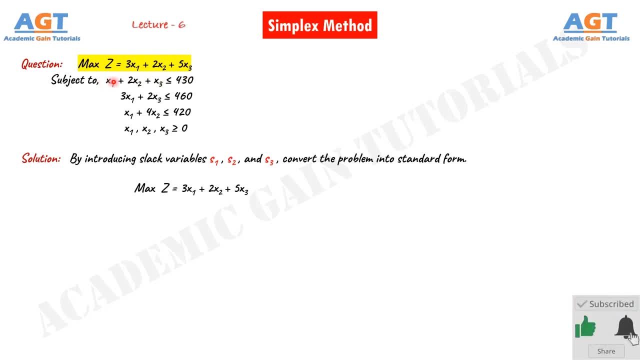 using slack variables. So for the first equation we will write: subject to x1, plus 2x2, plus x3, then leave some space and write: equals to 430.. For the second equation we will write 3x1, plus 2x3,, then leave some space and write: 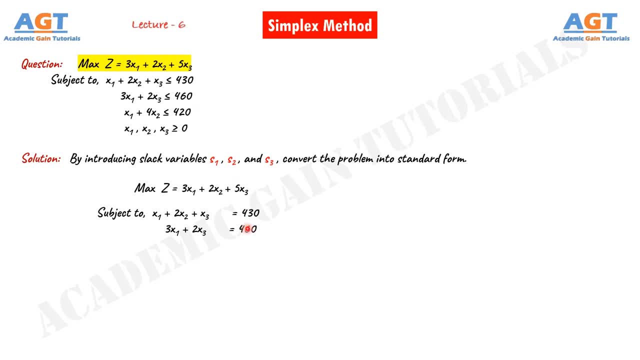 equals to 460.. For the third equation we will write: x1, plus 4x2, equals to 420.. Now on the first case. here we can see less than or equal to sign. that means this left: 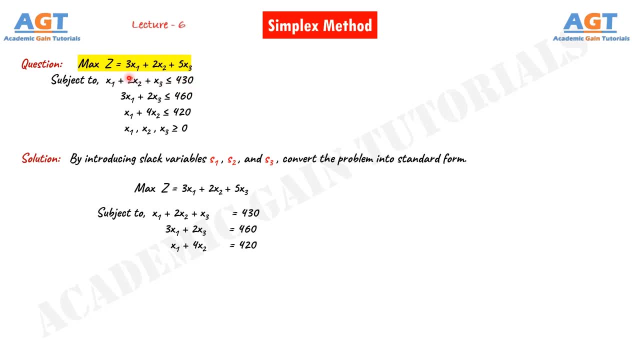 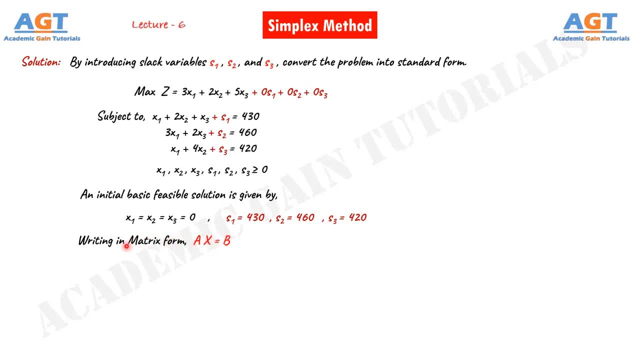 is the matrix form and we have to write the standard linear programming problem into this. a into X equals to be form. now, if we take a look at the constraints here, the cost of X 1 is 1. the cost of X 2 is 2. as we can see, the cost is written. 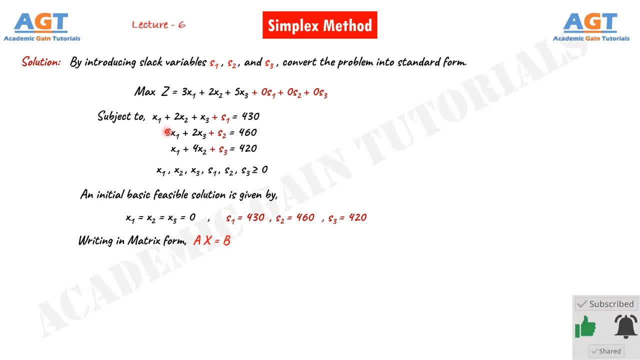 in front of X 2. similarly, the cost of X 1 over here is 3. so in the matrix form the letter a represents the cost of these six variables. again, the letter X in the matrix form represents these six variables and the letter B in the matrix. 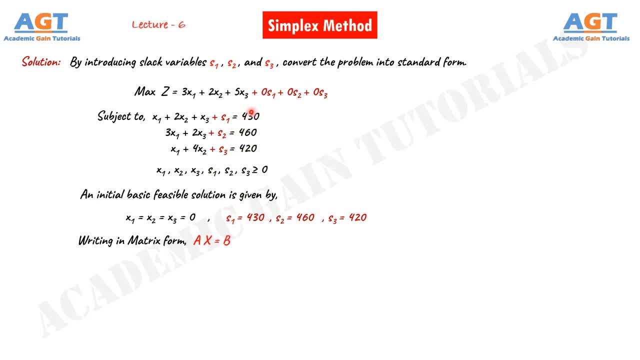 form represents the values we have here in the right hand side. so let's write the standard form LPP into matrix form in the headings at first. here we have written all the variables: X 1, X, 2, X 3, s, 1, s 2. and we have written all the variables X 1, X, 2, X, 3, s 1, s 2. and we have written all the variables X 1, X, 2, X 3, s 1, s 2 and s 3. now we will put the cost or the. 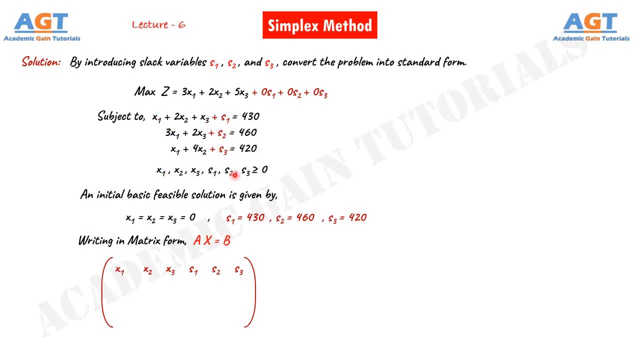 values of these variables from the standard LPP. here we can see that for the first constraint equation the value of X 1 is 1, the value of X 2 is 2, the value of X 3 is 1 and the value of s 1 is 1. so we put the values 1, 2, 1 and 1. 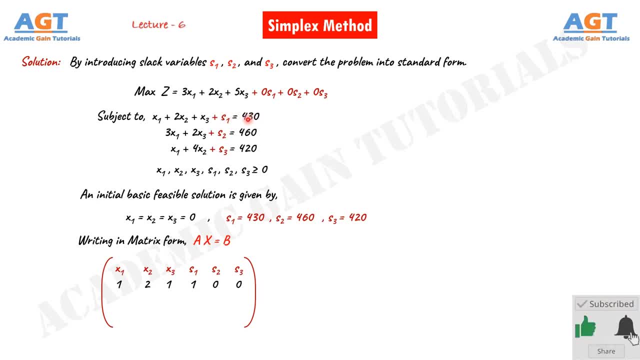 over here, since the first constraint equation does not have s 2 and s 3, so the value of s 2 and s 3 is 0. similarly for the second constraint equation, the value of x 1 is 3. there is no x 2 here, so value of x 2 is 0. the value of x 3 is 2. there is no s 1. 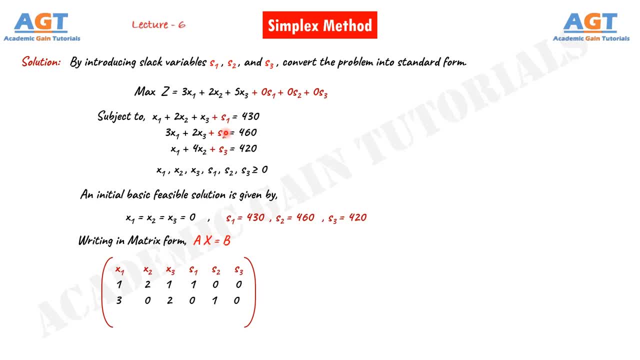 here. so value of s 1 is 0, the value of s 2 is 1 and since there is no s 3 here, so value of s 3 is 0. and for the third equation, the value of x 1 is 1, the value 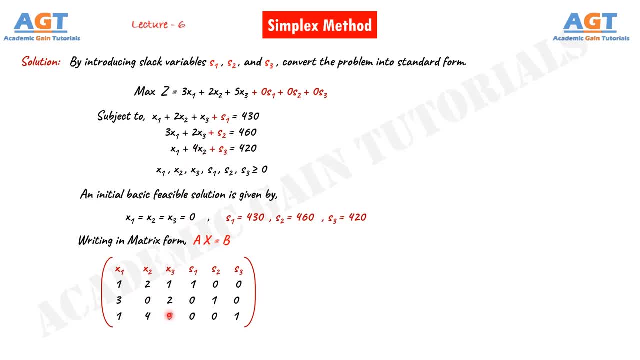 of x 2 is 4. there is no x 3, so the value of x 3 is 0. there is no s 1 and s 2 here, so value of s 1 and s 2 is also 0 and the value of s 3 is 1. so we have written the. 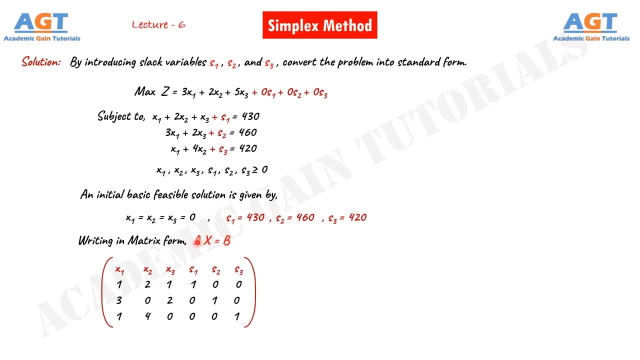 values of a in the matrix form. now for the values of X in the matrix form. we will write all the variables over here is the value of X. so we have written all the variables X, 1, X, 2, X, 3, s 1, s 2 and s 3 as the value of X. and finally, on the 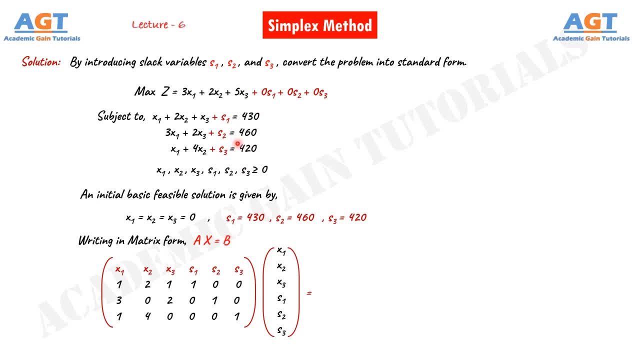 right hand side. we will write these values from the equations 430, 460 and 420. these are the values of B in the matrix form. so in this third step we have written the standard LPP into the matrix form, which is: ax equals to B and 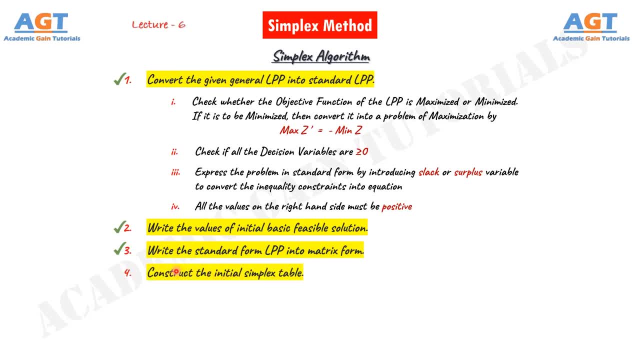 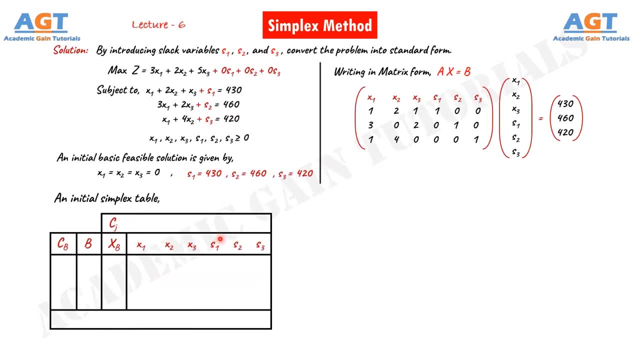 now, in step number four, we have to construct initial simplex table. so let's see how to make a simplex table. here we can see an initial simplex table. you have to make an initial simplex table exactly like this one and remember to leave some space on the right hand side of the table. we will use the space later. 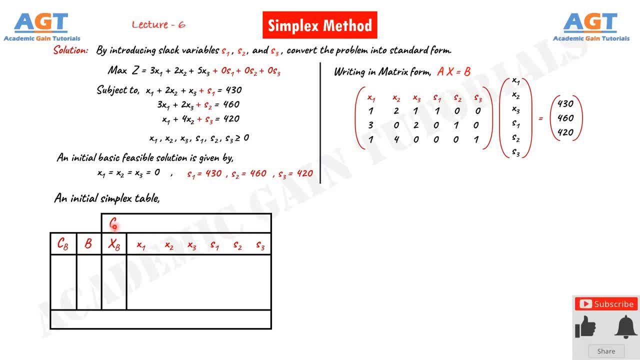 now the first row on the table is for CJ. to fill up this row for CJ, we will take a look at the objective function. here we have the objective function. here we have the objective function. we have six variables: X 1, X 2, X 3, s 1, s 2 and s 3, and in front of 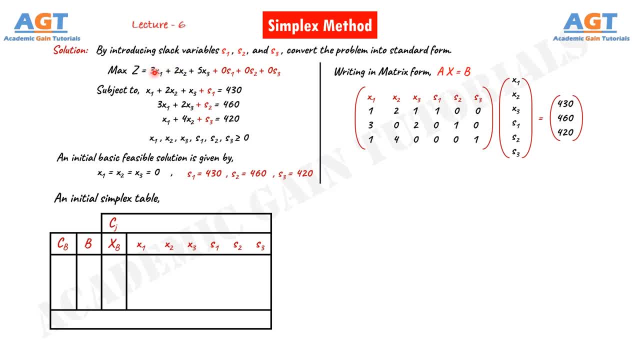 each variable. there is the cost of these variables: three, two, five, zero, zero and zero. we will write the cost of these variables from objective function to fill up the row for CJ over here. so we have written the costs: three for X 1, two for X 2, five for X 3, zero. 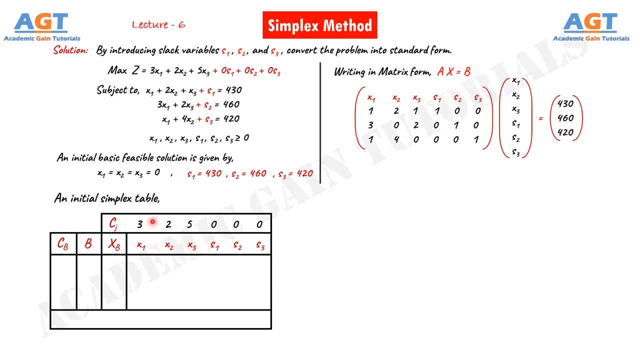 one, s 2 and s 3, so this row has been filled. now we will fill up the columns. the column B over here is the column for basic variables. when we will make the first initial table, the slack or surplus variables that we introduced into the problem earlier will be written in this. 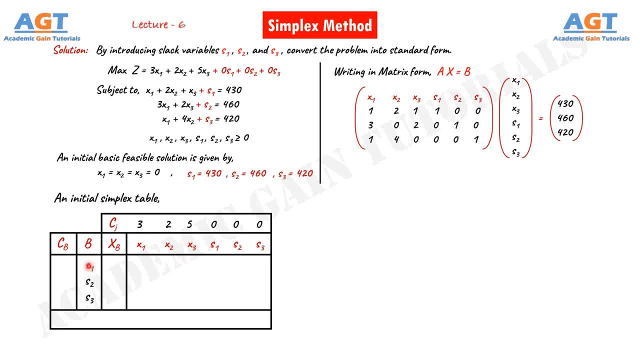 column B. so here we can see that we have three slack variables. so in the column B we will write the three slack variables s1, s2 and s3, And the column CB over here is for the cost of these basic variables in column B. so 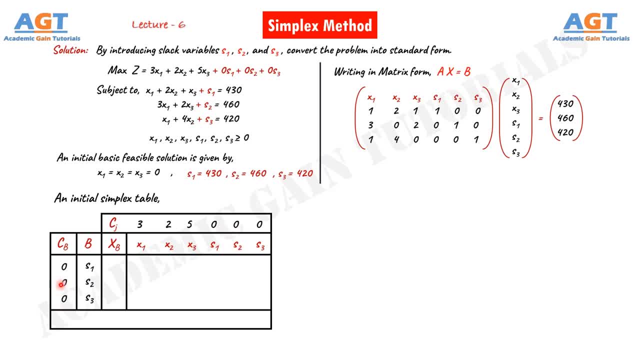 the cost of S1 is 0,. the cost of S2 and S3 are also 0.. Since this is the initial simplex table, the basic variables we write in this column B are all slack variables And we already know that the cost of slack and surplus variables is 0, so the value 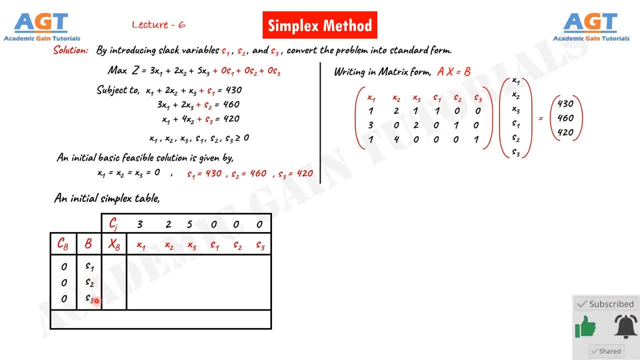 of CB will be 0 at first for all variables in the initial simplex table. Now in the column XP over here we will write the values from the right hand side of the matrix form. 430,, 460, and 420, are the values on the right hand side. 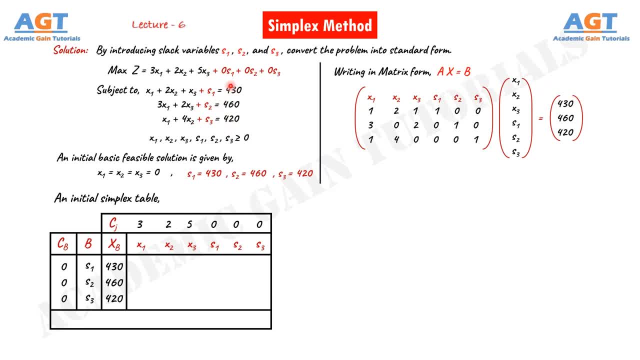 If you haven't made the matrix yet, you can take the values from right hand side of these equations also. So in the column XP we write the values from right hand side- Right hand side of the matrix- 430,, 460, and 420., 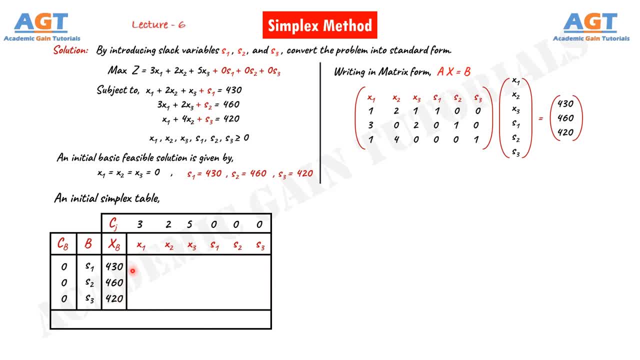 Now we have to fill up this region. we will put the values of the variables for these rows directly from the matrix over here. In the first row we have 1,, 2, 1,, 1,, 0, and 0.. 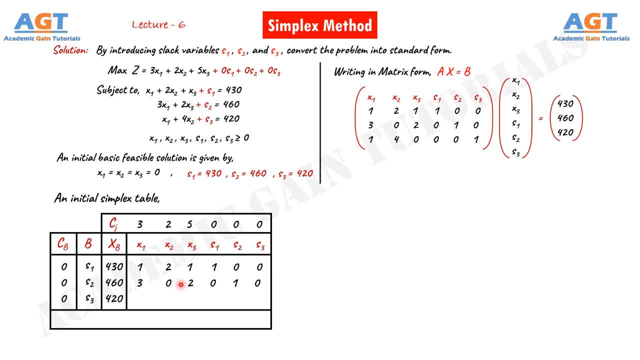 In the second row we have 3,, 0,, 2,, 0,, 1, and 0.. And in the last row we have 1,, 2,, 1,, 0, and 0.. 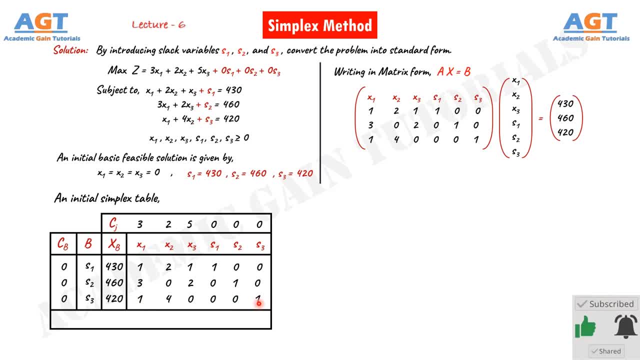 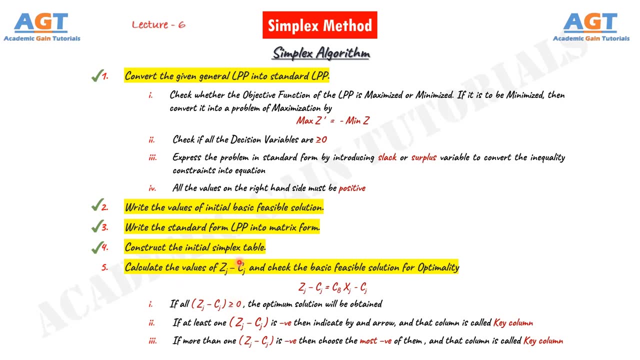 1,, 4,, 0,, 0,, 0, and 1.. The initial simplex table is now ready. So in this fourth step we have created the initial simplex table. Now the step number 5 is calculate the values of Zj minus Cj and check the basic feasible. 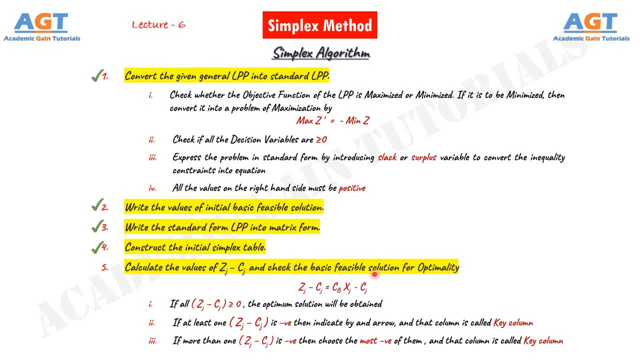 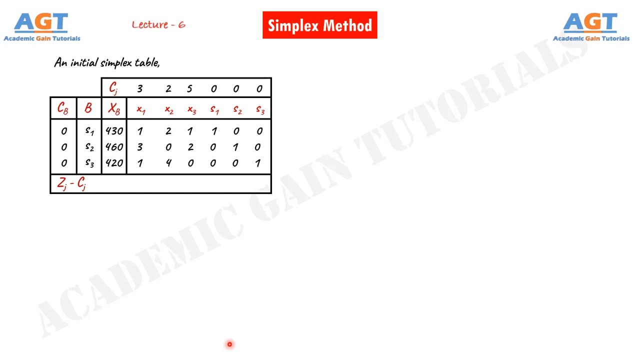 solution for optimality. So in this fifth step, we will at first calculate the values of Zj minus Cj Using this formula and following this steps. So let's find the value of Zj minus Cj at first. 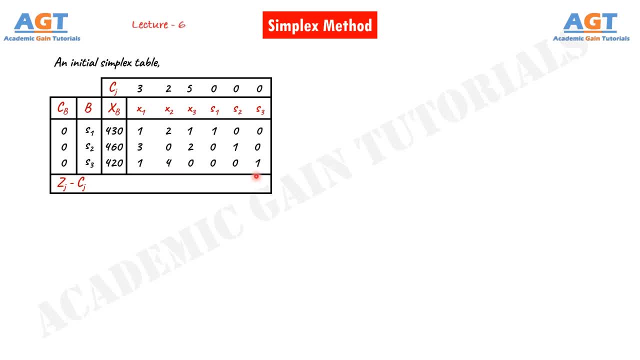 Now in the initial simplex table we have a row down here. this is the row for Zj minus Cj. For the calculation of Zj minus Cj, the general formula is: Zj minus Cj equals. 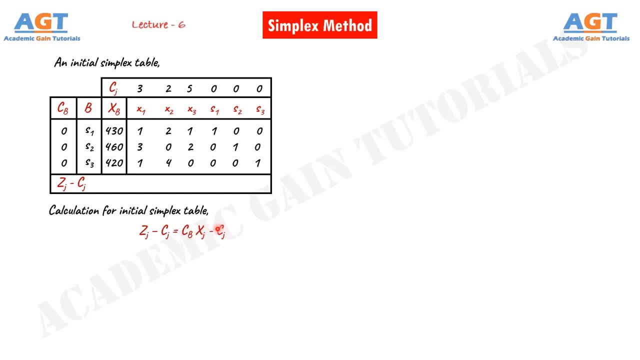 to Cb into Xj minus Cj. So this is a general formula and based on this general formula for the calculation of Z1, minus C1,, the formula will be: Z1, minus C1, equals to Cb into X1, minus. 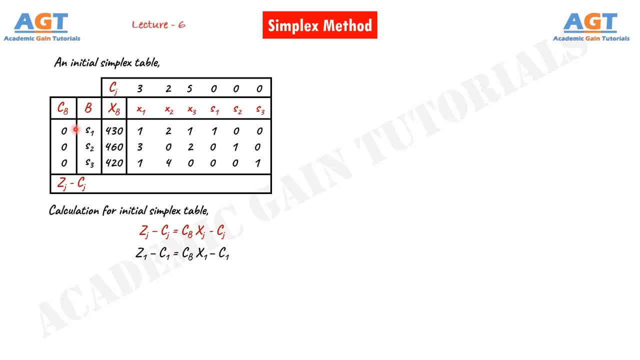 C1. Here, since this is the initial simplex table, the basic variables we write in this column B are all slack variables and we already know that the cost of slack or surplus variables is zero. So the value of Cb will be zero at first for all variables in the initial simplex table. 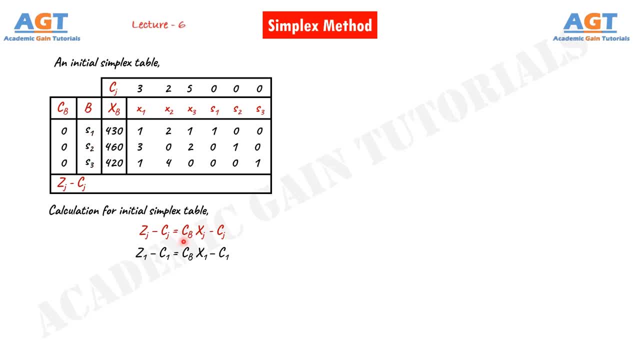 Now we have Cb into X1, the value of Cb is zero, zero and zero, and the value of X1 is 1,, 3, and 1, so the value of Cb into X1 will be zero into 1, plus zero, into 3, plus zero. 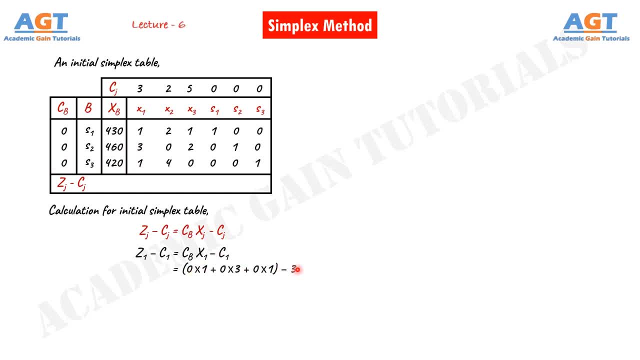 into 1, then give the minus sign And in the Cj row we can see the value of C1 is 3.. So we write 3 here and finally the value of Z1 minus C1 will be minus 3.. 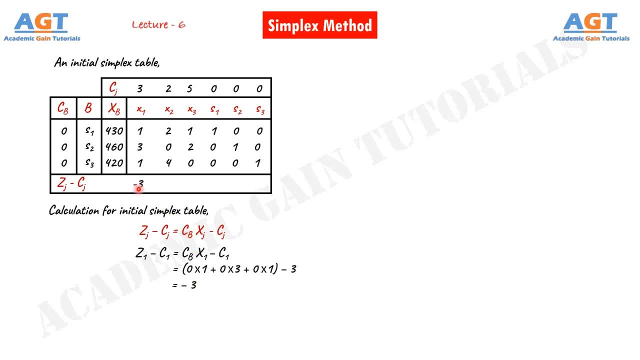 So in this row here we will write minus 3.. Now, in the same way, we will find out value of Z2, minus C2.. As we said earlier, since this is the initial simplex table, the basic variables we write. 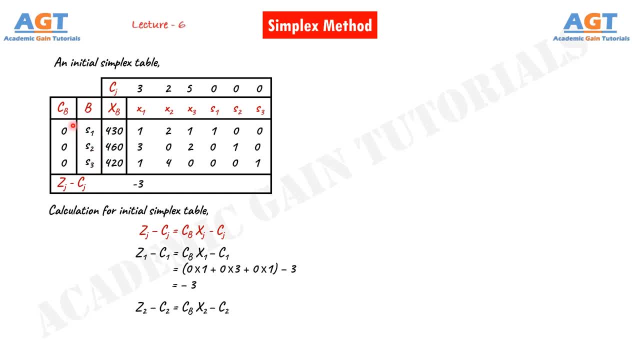 in this column B are all slack variables. So the value of Cb will be zero at first for all variables. So the value of Cb will be zero at first for all variables. So the value of Cb will be zero at first for all variables. 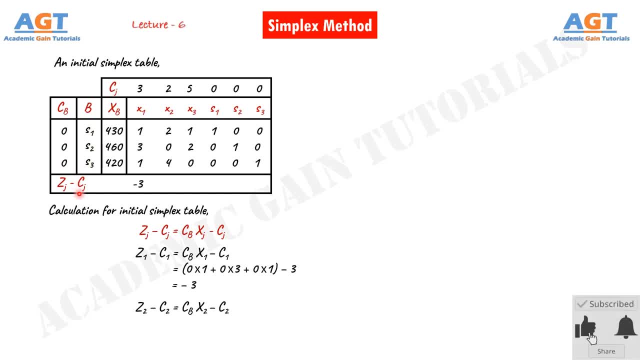 So in the initial simplex table the value of Zj minus Cj usually depends on Cj only, and the value of Zj minus Cj will be minus Cj. So we will find out value of Z2, minus C2.. 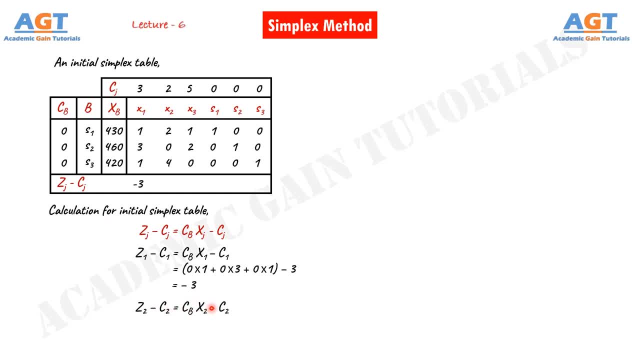 The formula will be Cb into X2, minus C2.. Here we will have zero into 2, plus zero into 0, plus zero into 4, minus. the value of C2 is minus C2.. 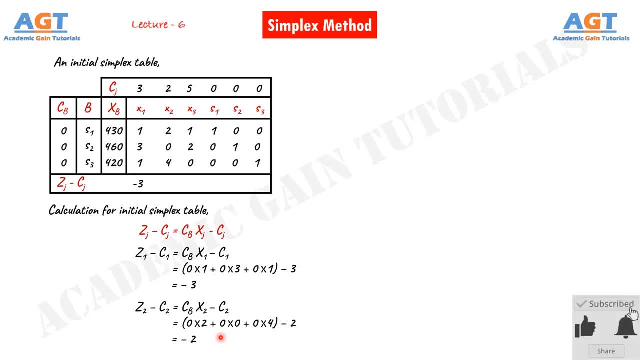 And finally, the value of Z2 minus C2 will be minus 2, so in this row here we will write minus 2.. Similarly we can calculate: the value for Z3 minus C3 will be minus 5.. 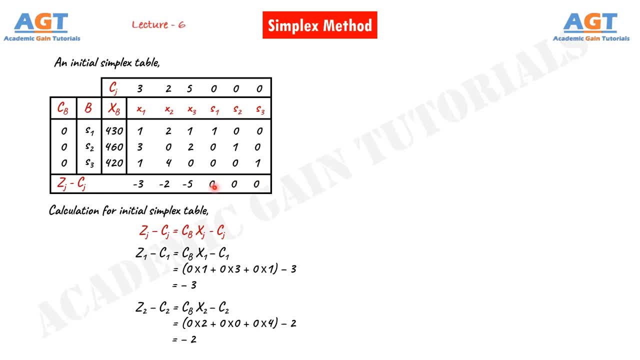 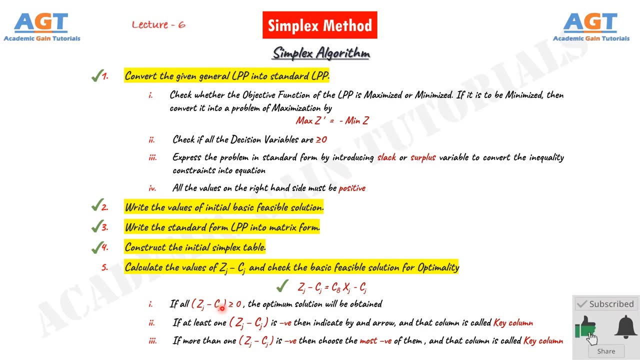 The value for Z4 minus C4 will be zero, and these two values will be also zero. So we have found out the values for Zj minus Cj using this formula. Now, after finding the values, the first condition is if all the values of Zj minus. 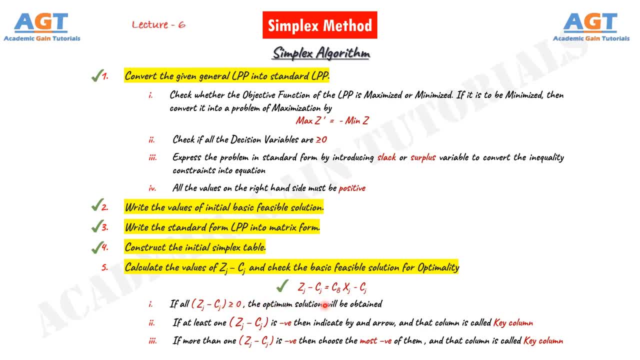 Cj are greater than or equal to zero, then the optimal solution will be obtained. So if the values of Zj minus Cj that we found out are either greater than zero or equal to zero, then we will obtain the optimal solution. 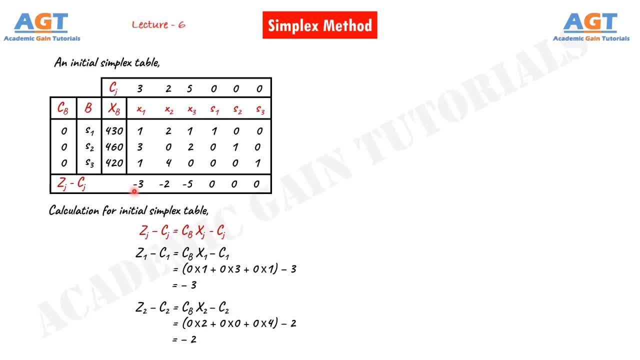 Now let's check over here. the values of Zj minus Cj are not greater than or equal to zero. Rather, we have negative values Here: minus 3,, minus 2,, minus 5, so all the values are not positive or equal to zero. 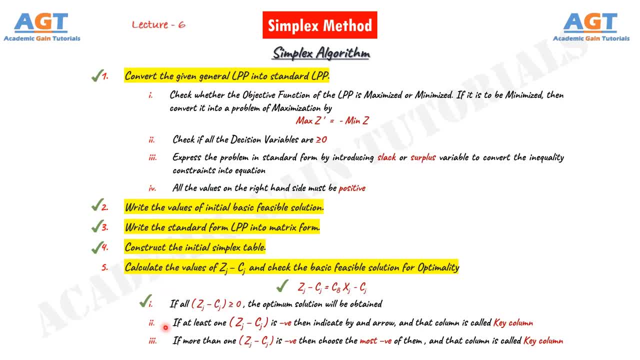 Thus the first condition is not fulfilled and we will not have the optimal solution here. So let's move to the second condition. The second condition says: if at least one value of Zj minus Cj is negative, then indicate by an arrow and that column will be called key column. 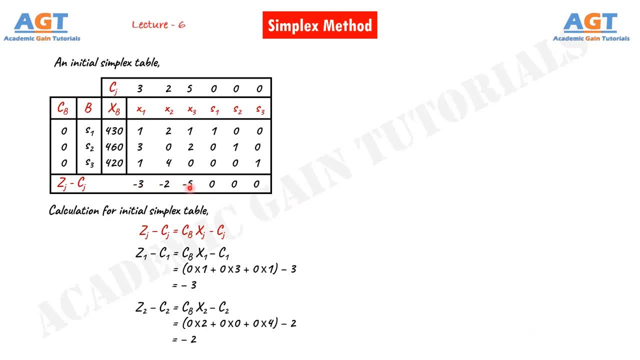 If we see in the table, We have three negative values of Zj minus Cj. If there was only one negative value, then we would indicate that negative value by an arrow and that column would be called key column, Since we have more than one negative value. the second condition is also not applicable. 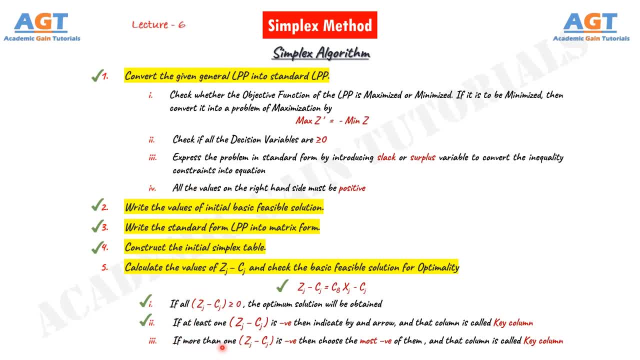 we will move to the third condition. The third condition says: if more than one or multiple values of Zj minus Cj are negative, then choose the most negative value of them, then indicate that most negative value by an arrow And that column will be called key column. 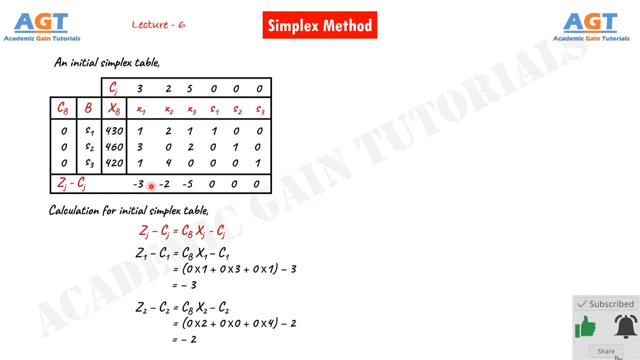 If we see in the table, We have three negative values of Zj minus Cj, minus 3, minus 2, minus 5, the most negative value among these three values is minus 5, we will now indicate this most negative value. 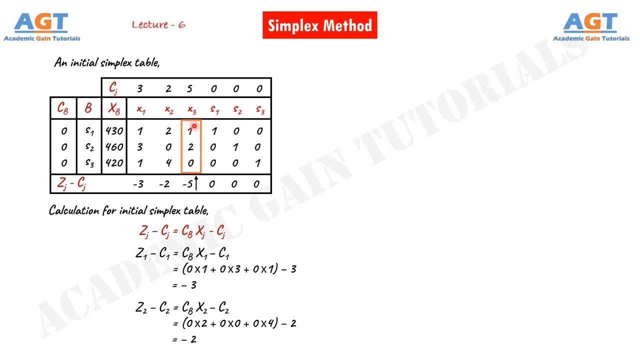 by an arrow and this corresponding column containing this arrow indicated value will be called key column. so this column x3 is the corresponding column to this value which we indicated with an arrow. Then, arrow, this column of x3 with the values 1,, 2, and 0, will be called the key column. 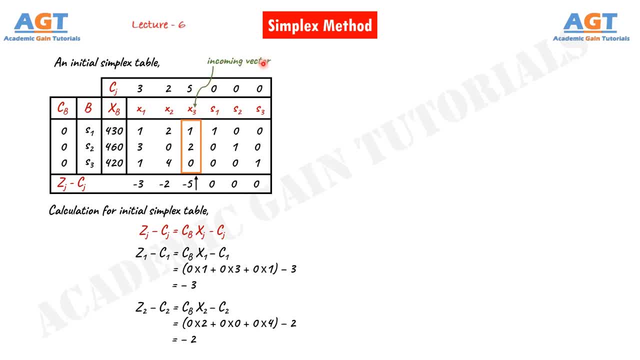 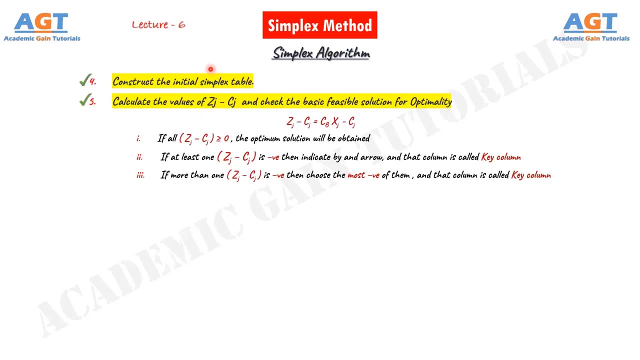 And x3 will be called incoming vector. So in step number 5, we have found out the values of Zj minus Cj. then, based on these three conditions, we found out the key column and the incoming vector. Now, in step number 6, we have to calculate the minimum ratio. 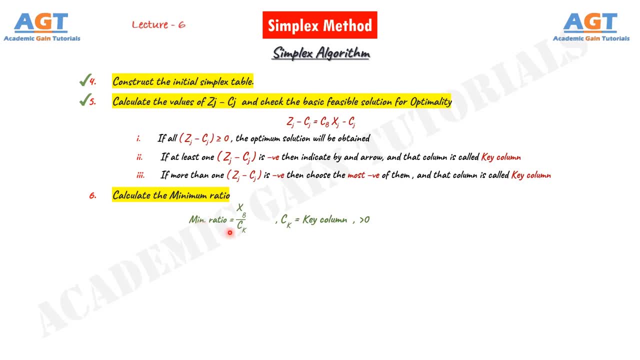 Here we have the formula for calculating minimum ratio. Here we have the formula for calculating minimum ratio. ratio equals to xp divided by ck. Here ck is the key column and the value of ck has to be greater than zero. So let's find out the minimum ratios. 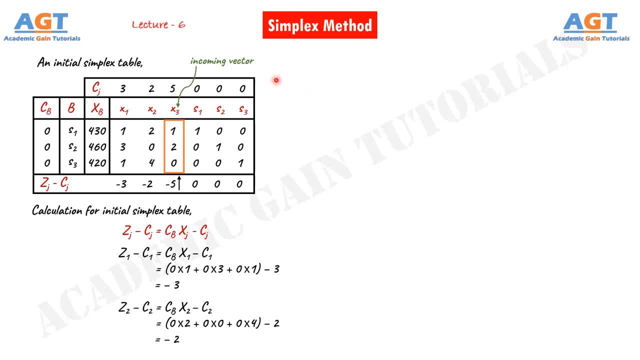 Now, on the right hand side of the initial simplex table, we had left some space. we will use that space for calculation of minimum ratio. When we made this initial simplex table, we did not make these column for minimum ratio at first, because after finding these values, 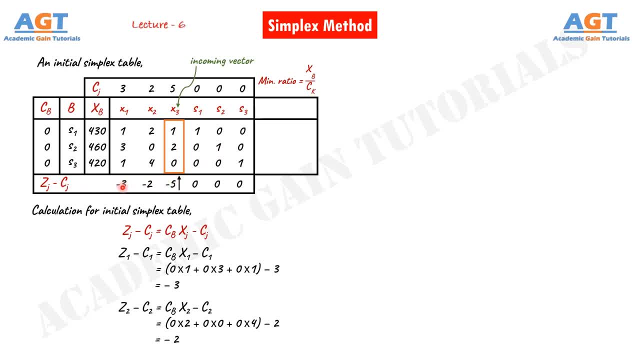 of zj minus cj. if we found out that all the values are greater than or equal to zero, then we would not have to calculate minimum ratio and we would not make the minimum ratio column. but here we have negative values of zj minus cj, so we need to calculate the minimum. 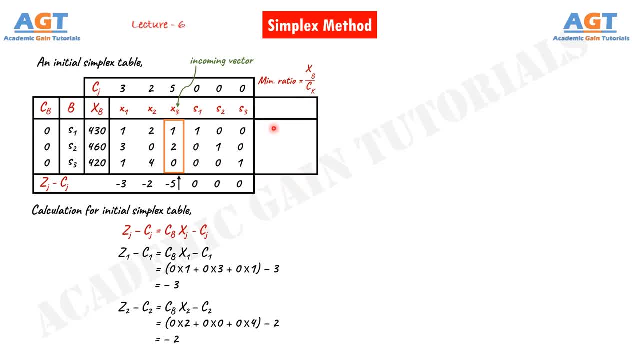 ratio. thus we made the minimum ratio column now. So the formula of minimum ratio is xp divided by key column. here the key column is this: x3 column. so we write the formula: minimum ratio equals to xp divided by x3.. 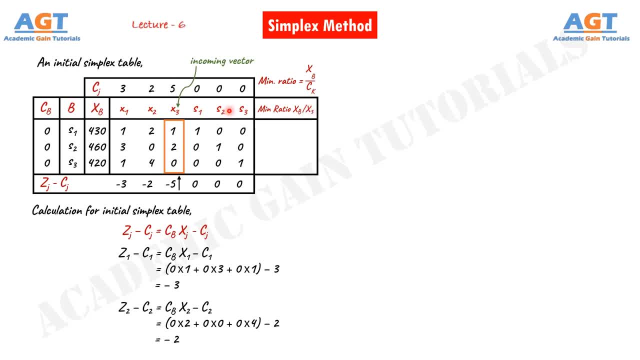 Here, x3 is the key column and the value of x3 has to be always greater than zero. if the value of ck is equal to zero or less than zero, then we will not find the minimum ratio for that row. Now for the first row. value of xp is 430,. 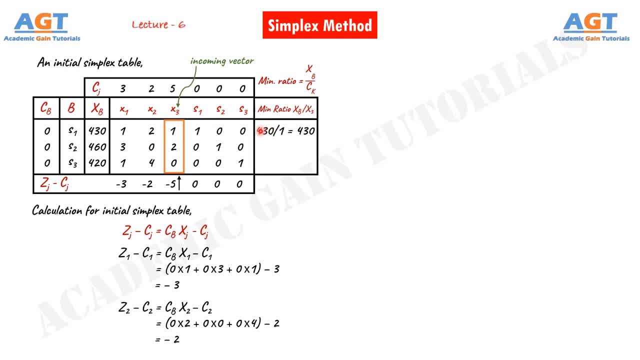 the value of x3 is 1, so the minimum ratio will be: 430 divided by 1 equals to 430.. For the second row, value of xp is 460 and the value of x3 is 2, so the minimum ratio. 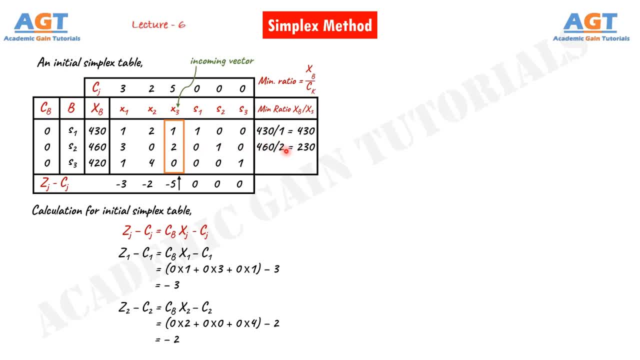 will be: 460 divided by 2 equals to 230.. And for the last row, value of xp is 420 and the value of x3 is 0.. Now, since the value of x3, or the key column, is 0 in this case, we will not calculate the. 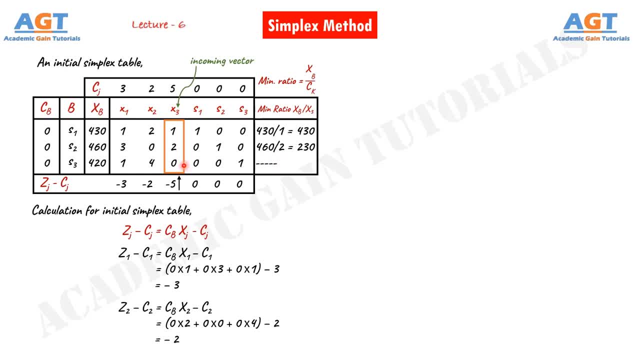 minimum ratio for this row. If we divided 420 by 0, it would ultimately give an undefined result. So we will not calculate the minimum ratio for this row, because x3 has to be greater than 0.. Now among 430 and 230.. 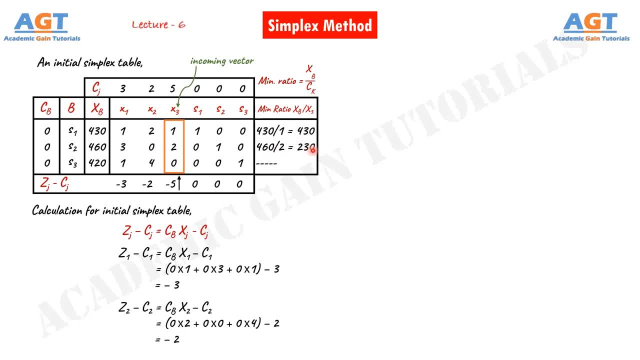 Now among 430 and 230.. The minimum value is 230, so we will indicate this minimum value, 230, by using an arrow like this. Now we made the first arrow here and this column x3 is the corresponding column to this. 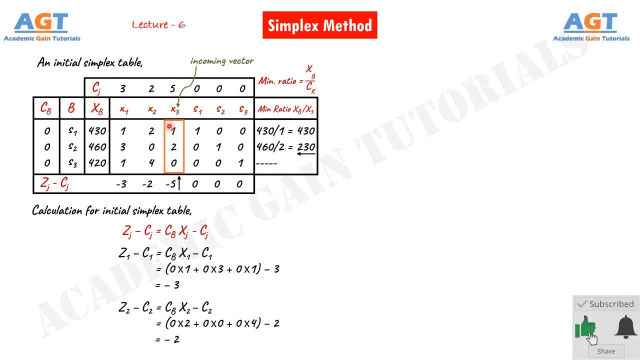 value which we indicated with the first arrow. This column of x3 is called the key column And x3 is called incoming vector. Now, in the case of minimum ratio, when we got the minimum value from minimum ratio, we also indicated this minimum value with an arrow. 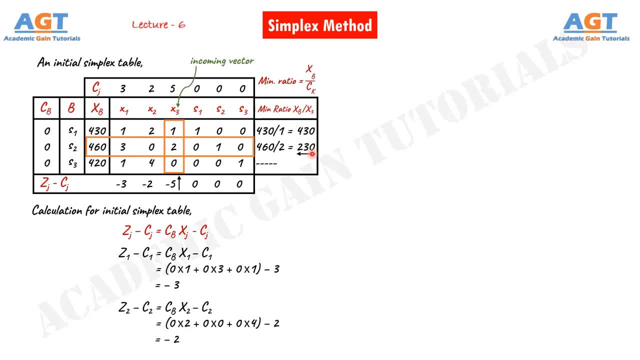 And this row is the corresponding row to this value which we indicated with this arrow. So this corresponding row is called the key row And the variable in front of the key row is s2.. So this variable, s2, is called outgoing vector. 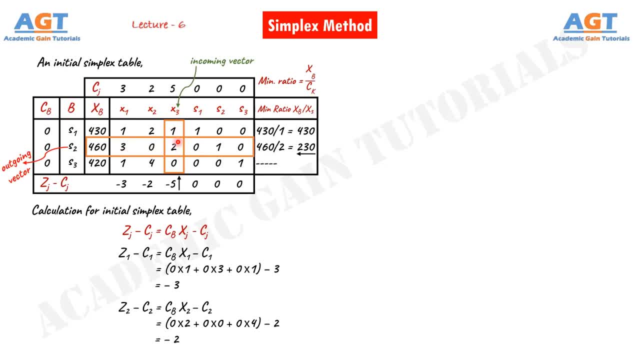 And this common element between this key row and key column is called key element. Here, 2 is the common element between key row and key column, So this key row is called key column, So 2 is the key element. So in step number 6, we have found out the minimum ratios. 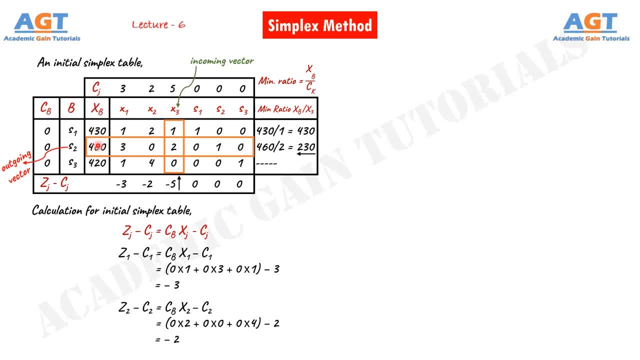 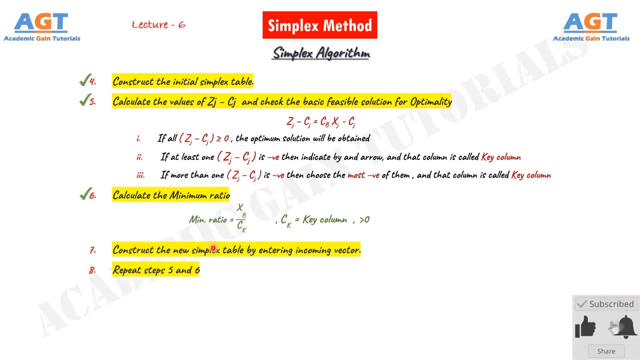 Then, based on the minimum value, we found out the key row, the outgoing vector and the key element. Now, in step number 7, we have to construct the new simplex table by entering incoming vector, And after that we will repeat step number 5 and 6.. 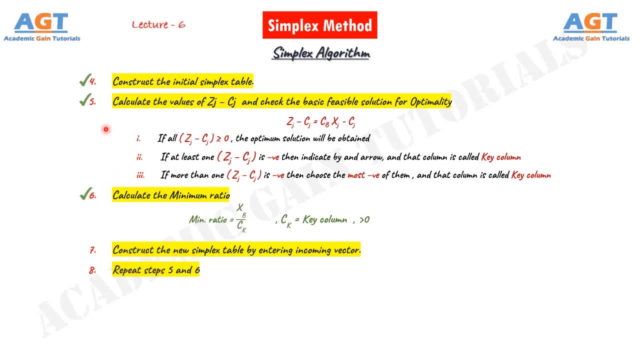 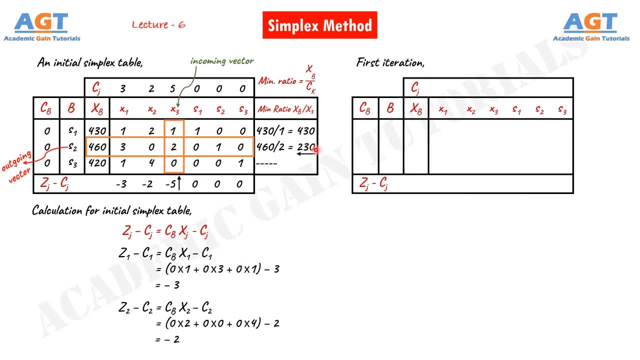 So we have to repeat the step number 5, and step number 6 again after constructing the new simplex table. So, moving forward here, we have made a new simplex table. In the heading we have written 1st iteration. So this is the first iteration, simplex table. 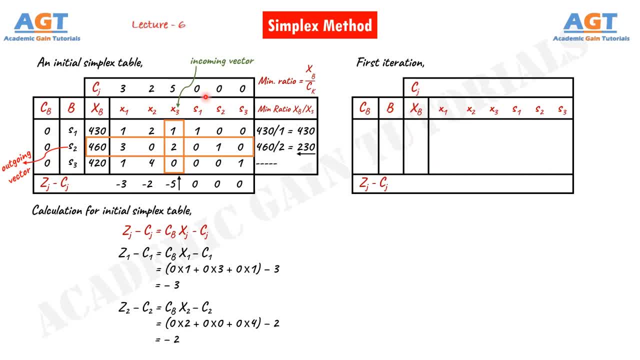 We have constructed this new simplex table exactly like the first table. When we filled up the values for the initial simplex table, we had easily looked at the matrix and filled the values from the matrix to the initial simplex table without much calculation. In this new simplex table we have to calculate each value to fill up the table. 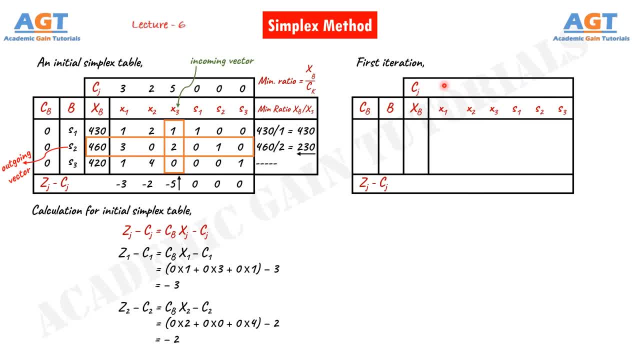 The value of cjRow will remain same because the cost of the objective function has remained same. So we will copy and write the value of cj from the table number 1 to this new table. Here we will write 3,, 2,, 5,, 0,, 0, and 0,, as the cost will remain same. 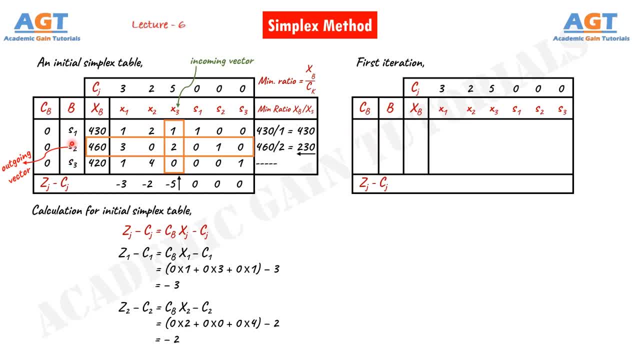 In the basic variable in the first table we had s1,, s2, and s3. Here, s2 is the outgoing vector and in place of s2, the incoming vector is x3. So in place of s2, we will write x3. 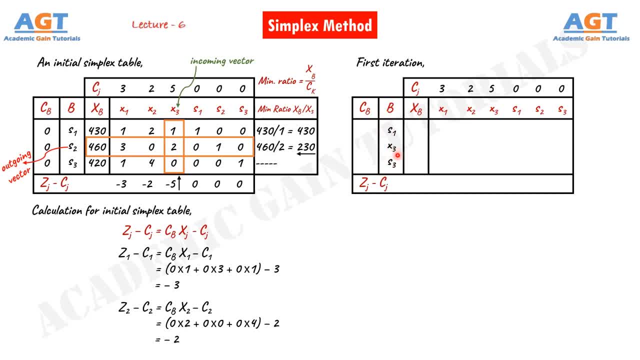 Here we have written the basic variables s1, x3, and s3.. So we have replaced s2 by x3.. Now we will write the cost of these variables here. So the cost of s1 is 0. 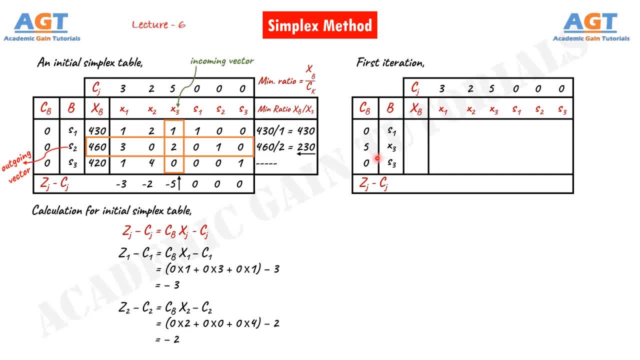 The cost of x3 is 5. And the cost of s3 is 0. Now, starting from xp, we have to fill up the rest of this table by doing some calculations, And we will do the calculations by looking at table number 1.. 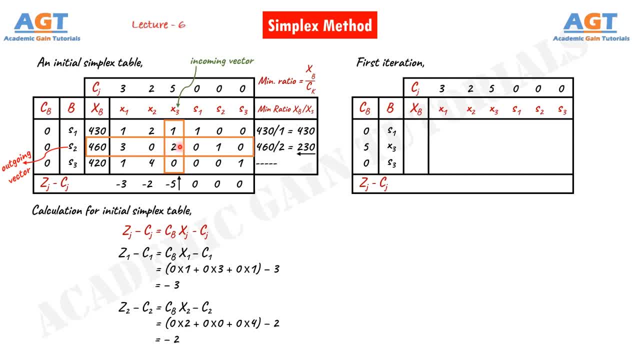 Now 2 is the key element here. This key element has very important role in doing the calculations. Now, this key element is in second row, So we will divide all the values of the second row by this key element. In other words, this key element is in second row. 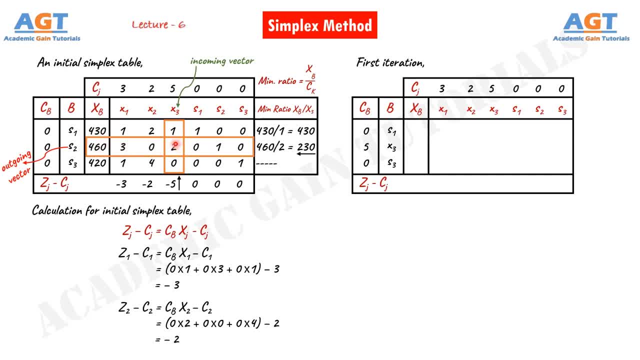 We will divide all elements of the key row by the key element. We will divide 460 by 2,, divide 3 by 2, similarly the other elements also. So when we divide 460 by 2, in the new table we will write 230 in the place of 460.. 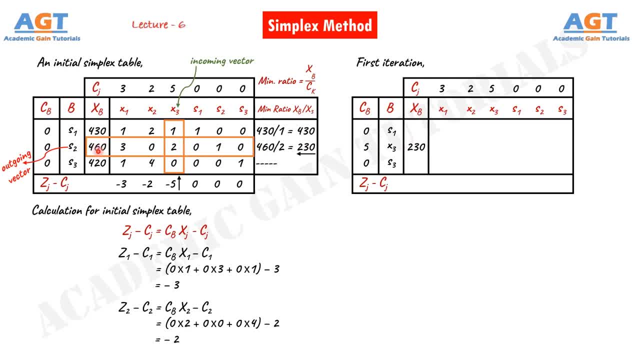 We are replacing the second row in the old table, So we will write the new values in the second row of the new table. So here we will have 3 divided by 2.. Then 0 divided by 2.. 2, which gives us 0,. 2 divided by 2,, which gives us 1, then we will have 0, 1 divided. 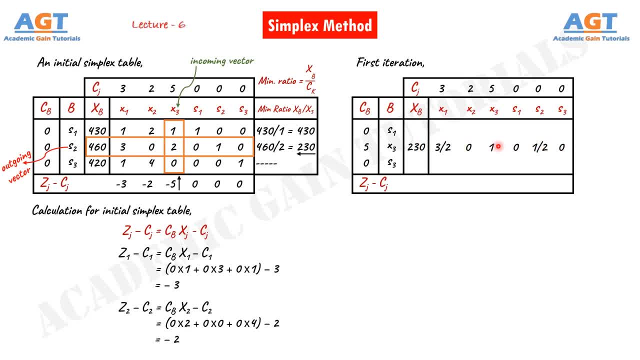 by 2, and 0.. So why are we doing this? If you observe carefully, in table number 1, the basic variables were s1, s2, and s3.. If you observe the values of s1 column, here we have 1,, 0,, 0,. in the s2 column, here we 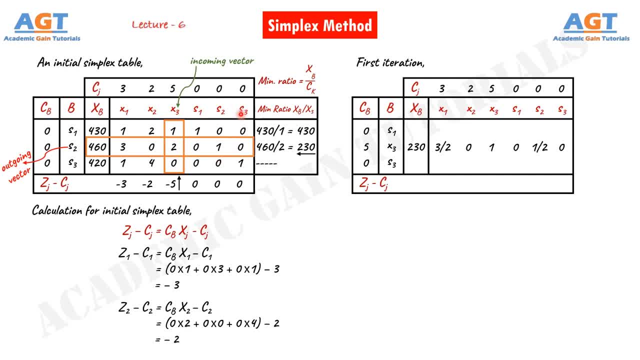 have 0, 1, 0, and in the s3 column here we have 0, 0, 1,, so this forms an identity matrix. The basic variables are written serially as s1,, s2, and s3, and if the s1,, s2, and s3 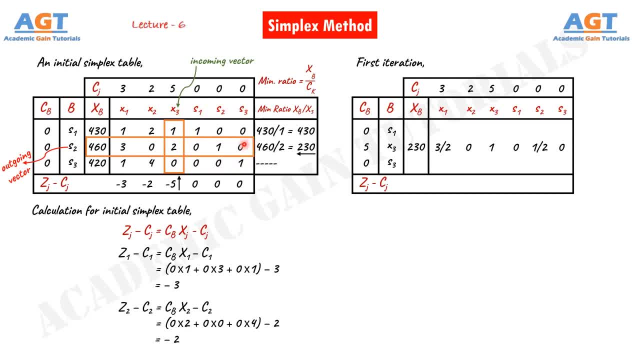 columns are arranged in the same serial, we get an identity matrix like this Now in the table 2 also, the basic variables are s1, s3, and s3.. If the s1,, s3, and s3 columns are arranged in the same serial, we should get an identity. 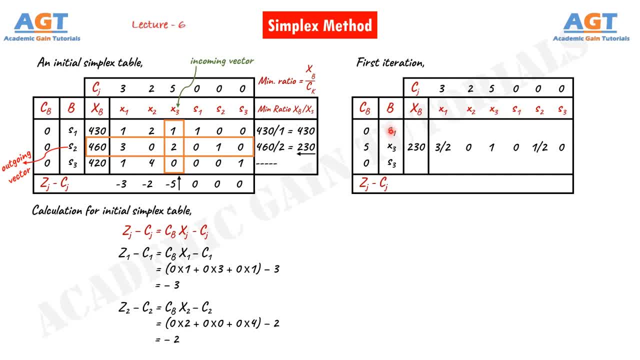 matrix: The first basic variable is s1,. in the first table we saw the value of the first basic variable s1 column was 1, 0, 0,. so in new table in the first basic variable, s1 column. 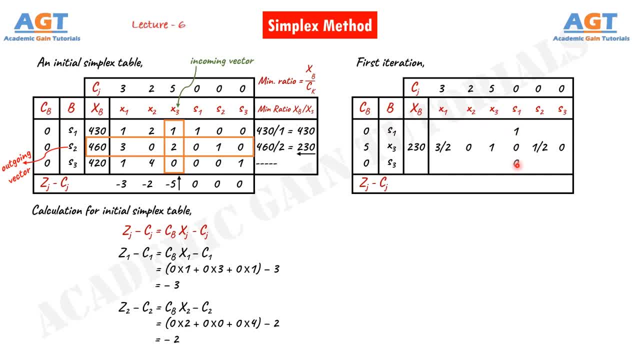 we will write 1, 0, 0.. Now the second basic variable is s3,. in the first table we saw the value of the second basic variable, s2 column was 0, 1, 0,. so in new table, in the second basic variable, 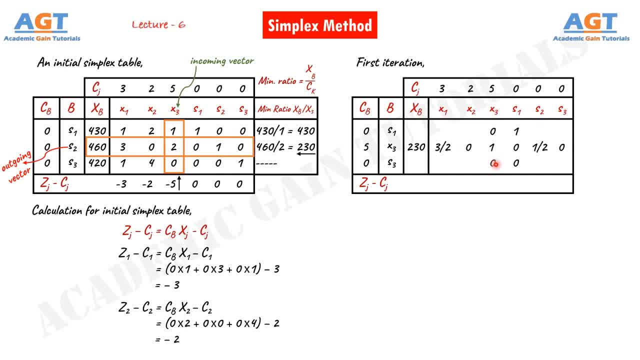 s3 column we will write 0,, 1,, 0, and the third basic variable is s3.. In the first table we saw the value of the third basic variable, s3 column was 0, 0, 1,. 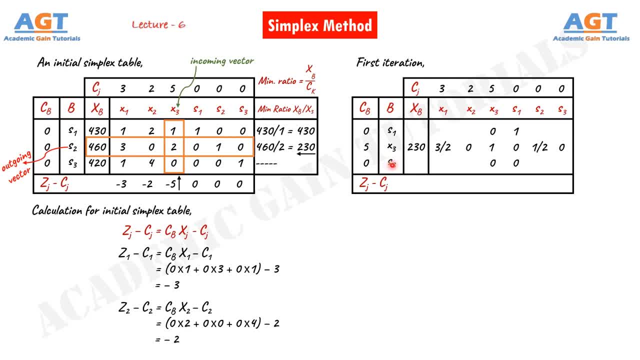 so in new table in the third basic variable, s3, column, we will write 0,, 0,, 1.. Now If we arrange the columns of S1,, X3, and S3 serially, we will get an identity matrix form like this one: 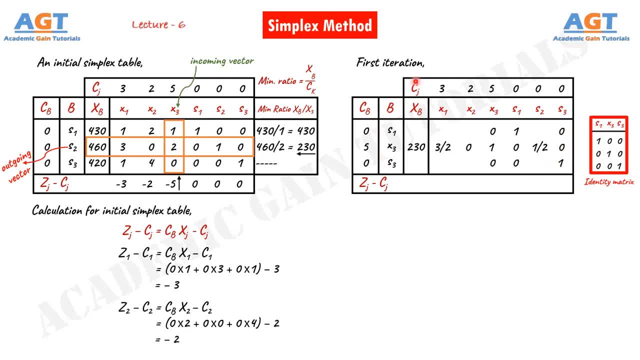 In this lecture we will see two methods of forming this table. We are learning one method now and if we require a new simplex table for finding the values, then in the second iteration table we will see another method of forming this table. You can solve using any one method that seems easier to you. 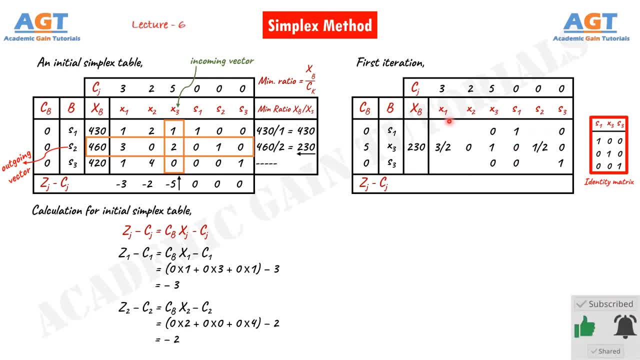 So in this first method we have formed the table and filled some portion of it, but we don't know the values to fill up these empty spaces. So to find out these remaining values we have to look back in the first table. 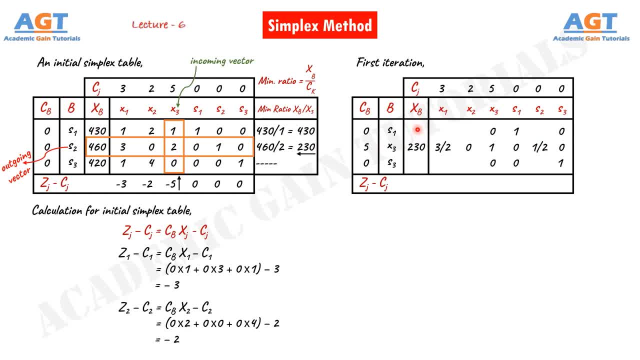 Let's find out the value for this position at first In the table number 1, in this position we have 430.. So we go to table number 1, then we will directly cross, multiply 430 with the key element. Here we have 430. 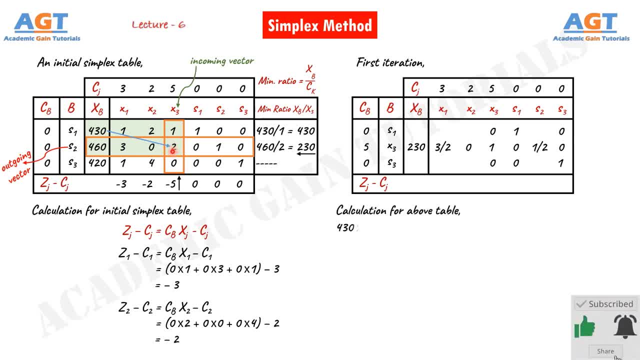 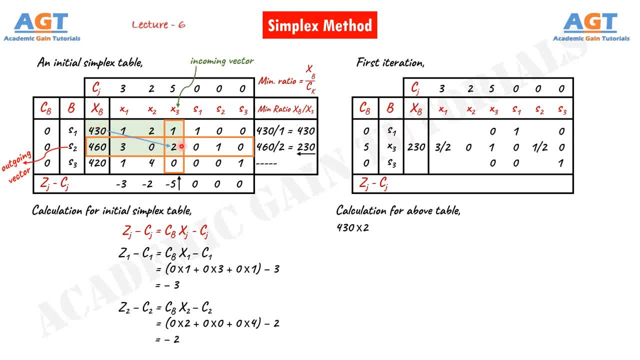 So we directly multiplied 430 by key element 2. And then we can see that here we have 460, and here we have 1.. If we multiply 460 and 1, it will form a cross diagonally. We multiplied 430 with 2, and we will multiply 460 with 1 over here. 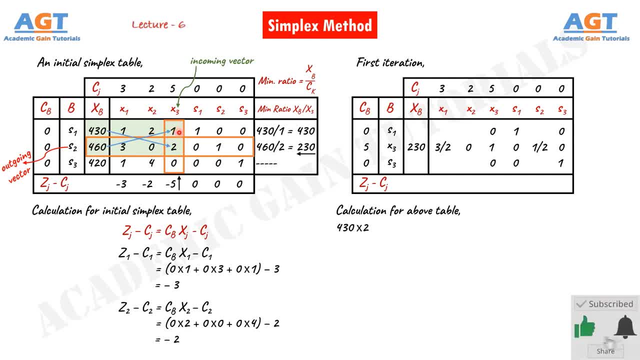 So it will be a cross diagonally. So in calculation we write 430 multiplied with 2, minus 460 into 1.. Then we will divide this whole thing by the key element. Here the key element is 2.. So we divide the whole expression by 2.. 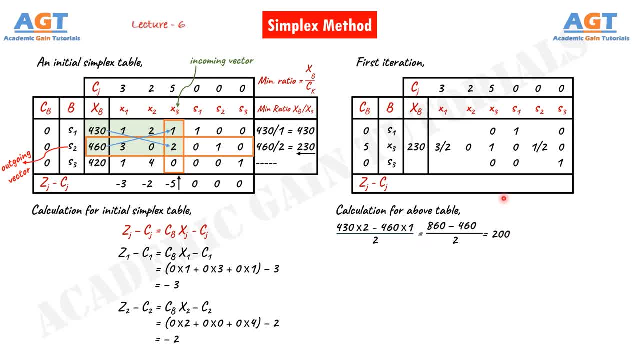 And finally we will get a value of 200.. We were finding this value for this position, So we will write 200 in this position. Now we will find out the value for this position in the table number 1.. In this position we have 420. 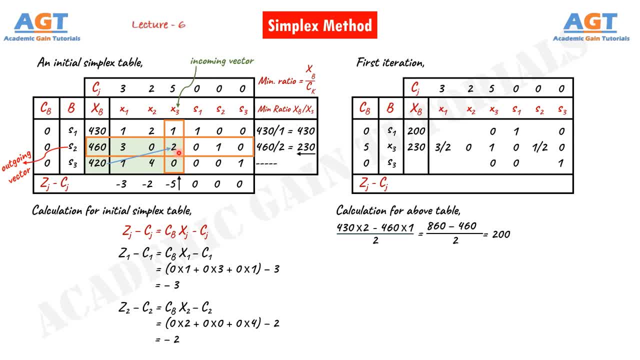 We will directly cross, multiply 420 with the key element. Here the key element is 2.. So we will multiply 420 with 2. And then we can see that here we have 460, and here we have 0.. 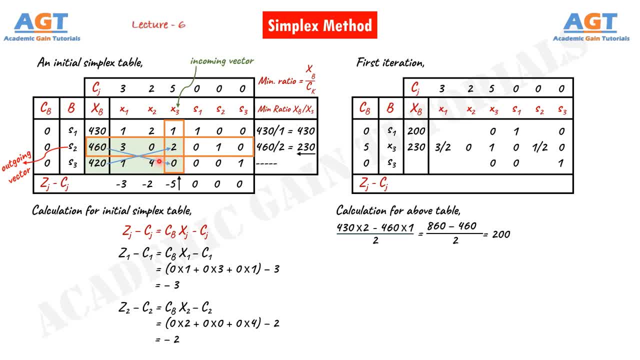 If we multiply 460 and 0, it will form a cross diagonally. We multiplied 420 with 2, and we will multiply 460 with 0 over here, So it will be a cross multiplication. So in calculation we write 420 multiplied with 2, minus 460, into 0. 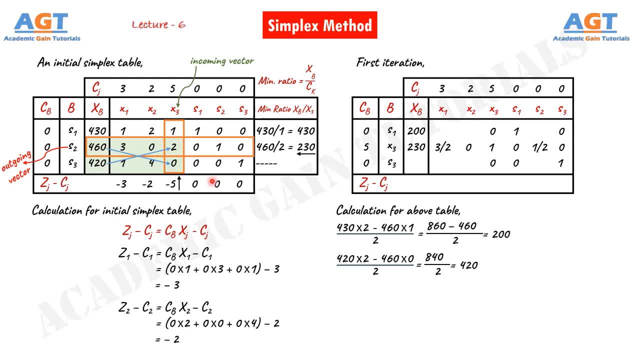 Then we will divide this whole thing by the key element. Here the key element is 2.. So we divide the whole expression by 2. And finally we will get a value of 420.. We were finding this value for this position. 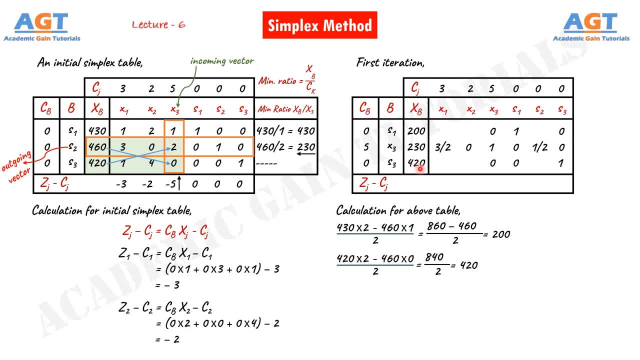 So we will write 420 in this position. Similarly, we will find out the value for this position In the first table. in this position we have 1.. We will directly cross multiply 1 with the key element 2.. Remember that we need to find this position in new table. 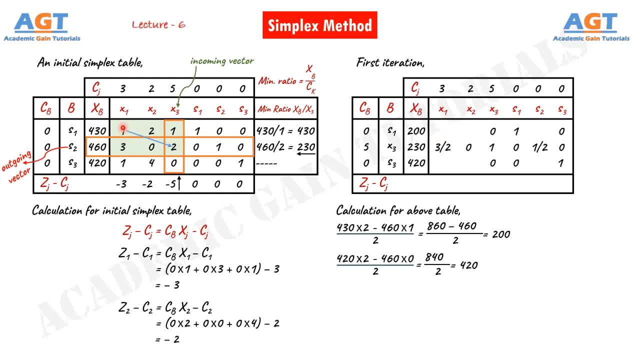 So we will multiply this value with key element first. Then we will multiply the other two corner values of the imaginary rectangle. that makes a perfect cross with this one. So we will cross, multiply 1 with 2.. We can see that here we have 3, and here we have 1.. 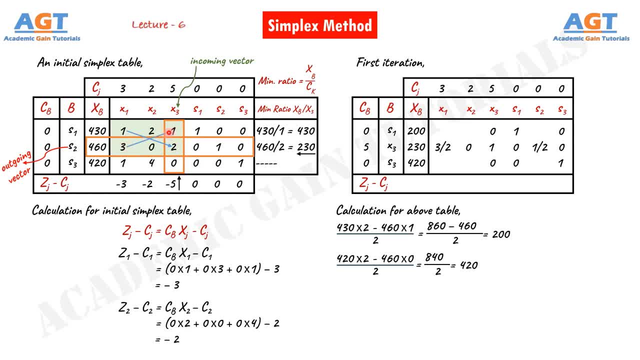 If we multiply 3 and 1. It will form a cross diagonally. So in calculation we write 1 multiplied with 2, minus 3 into 1.. Then we will divide this whole thing by the key element 2.. 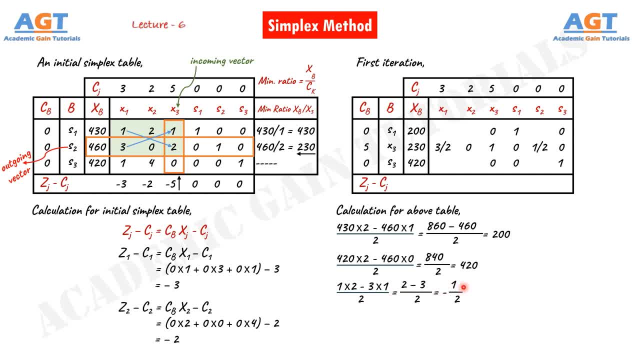 And finally, we will get a value of minus 1 by 2.. We were finding this value for this position, So we will write minus 1 by 2 in this position. Similarly, we will find out the value for this position. 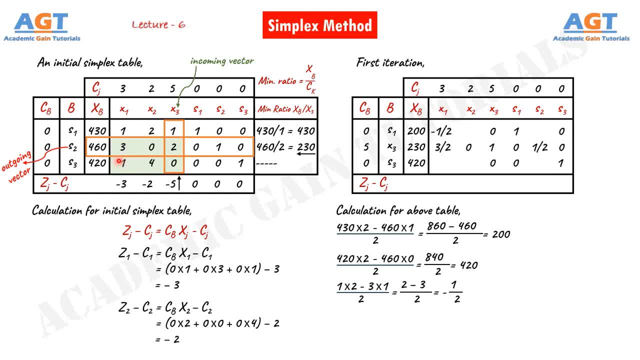 In the first table. in this position we have 1. We will directly cross, multiply 1 with the key element 2. We can see that here we have 3, and here we have 0. If we multiply 3 and 0.. 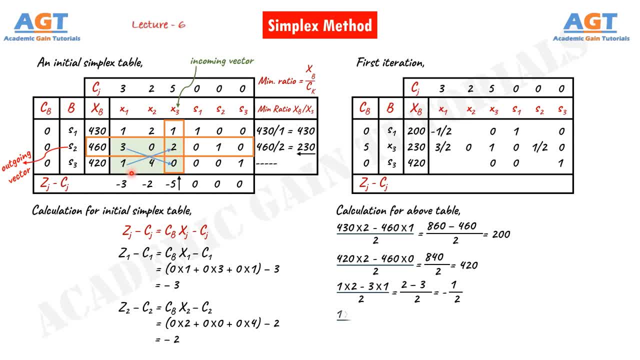 It will form a cross diagonally. So in calculation we write 1 multiplied with 2, minus 3 into 0. Then we will divide this whole thing by the key element 2. And finally we will get a value of 1.. 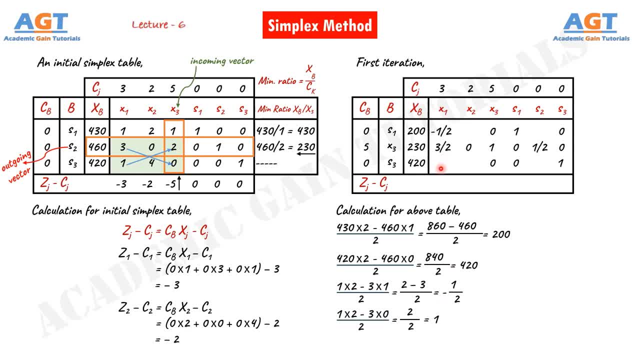 We were finding this value for this position, So we will write 1 in this position. Similarly, we will find out the value for this position In the first table. in this position we have 2.. We will directly cross multiply 2 with the key element 2.. 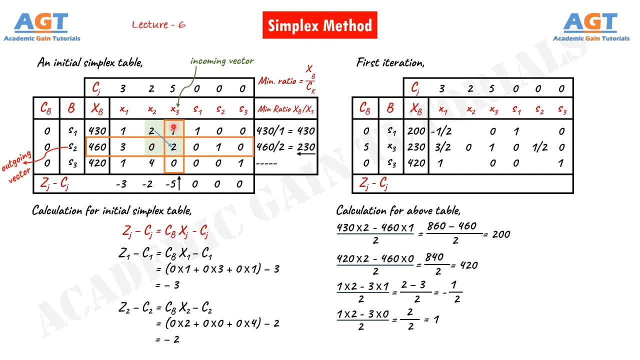 We can see that here we have 0, and here we have 1.. If we multiply 0 and 1. It will form a cross diagonally. So in calculation we write 2 multiplied with 2, minus 0 into 1.. 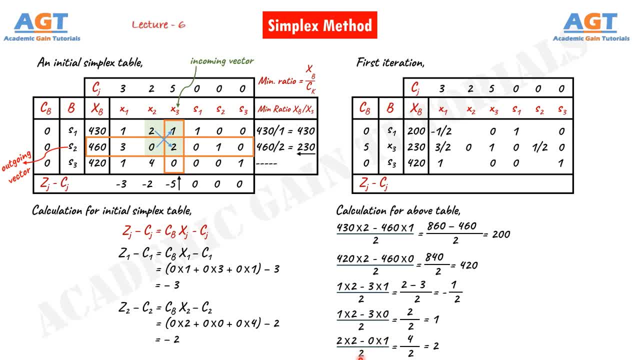 Then we will divide this whole thing by the key element 2.. And finally, we will get a value for this position. We will get a value of 2.. We were finding this value for this position, So we will write 2 in this position. 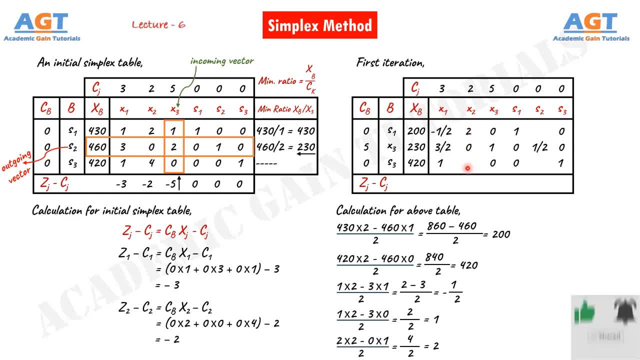 Now we will find out the value for this position In the first table. in this position we have 4.. We will directly cross, multiply 4 with the key element 2.. We can see that here we have 0, and here we have 0.. 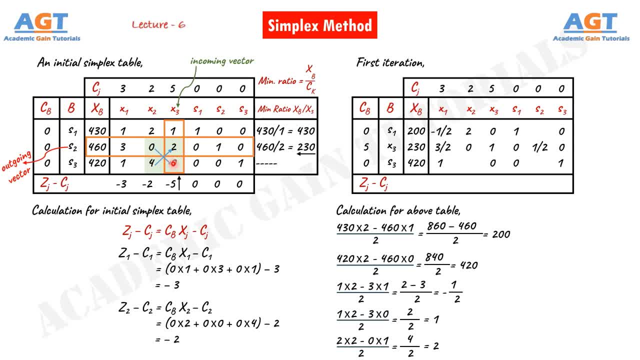 So we will multiply 0 and 0. It will form a cross diagonally. So in calculation we write 4 multiplied with 2, minus 0 into 1.. Then we will divide this whole thing by the key element 2.. 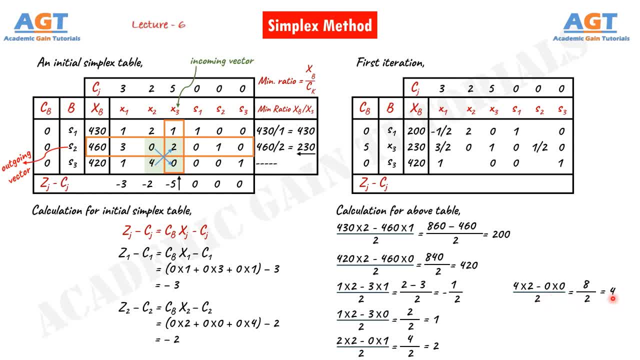 And finally we will get a value of 4.. We were finding this value for this position, So we will write 4 in this position. We have 2 more empty spaces left. We will find out the value for this position now. 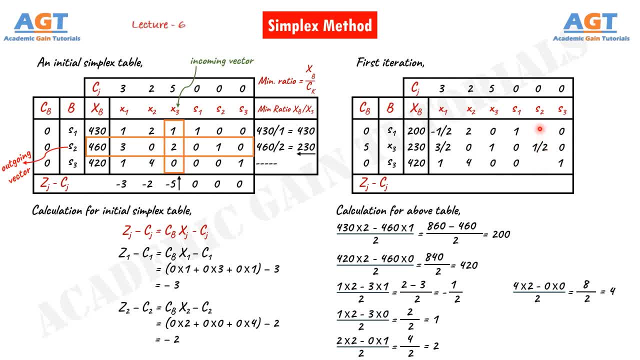 In the first table. in this position we have 0.. We will directly cross multiply 0 with the key element 2.. We can see that here we have 1, and here we have 1.. So we will divide this whole thing by the key element 2.. 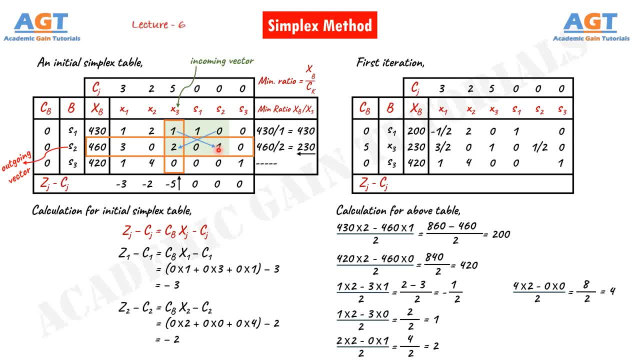 Here we have 1,, so we will multiply 1 and 1, it will form a cross diagonally. so in calculation we write 0 multiplied with 2, minus 1 into 1, then we will divide this. 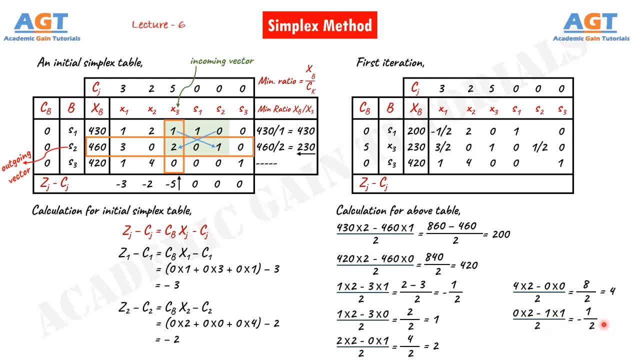 whole thing by the key element 2, and finally we will get a value of minus 1 by 2,. we were finding this value for this position, so we will write minus 1 by 2, in this position. 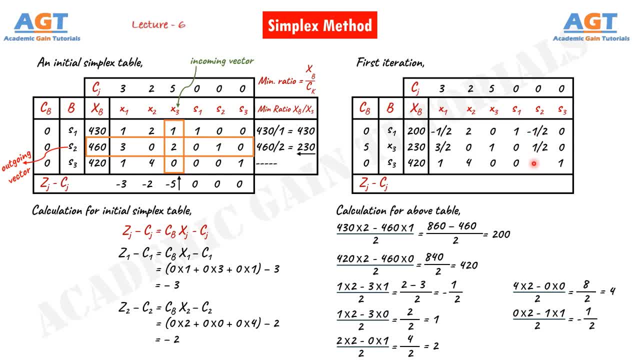 So this is the last empty space in this table. we will find out the value for this position now in the first table. in this position we have 0,. we will directly cross, multiply 0, with the key element 2, we can see that here we have 0, and here we have 1,. so we 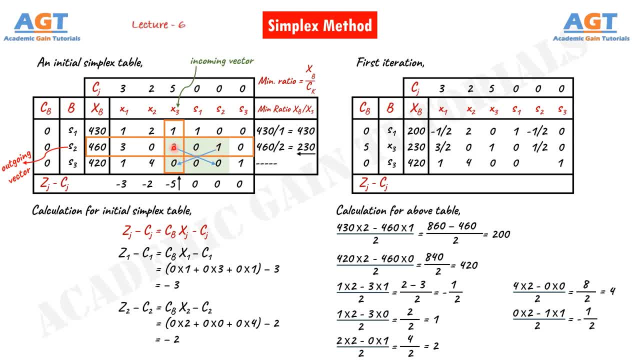 will multiply 0 and 1, it will form a cross diagonally. so in calculation we write 0 multiplied with 2, minus 0 into 1, then we will divide this whole thing by the key element 2, and the value is 0, we were finding this value for this position, so we will write: 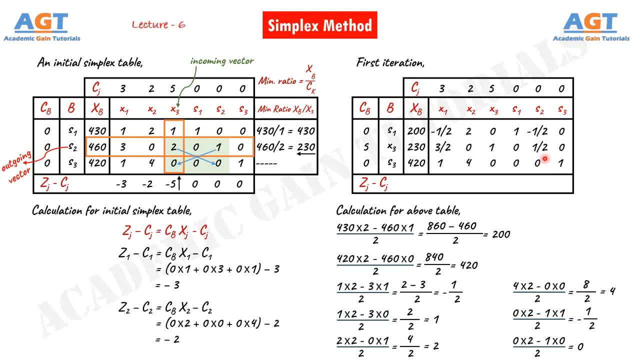 0 in this position. So we have prepared the simplex table for the first iteration. we have filled all the values in this first iteration table. Now we will find out the values for Zj minus Cj and fill up this last row. we will find. 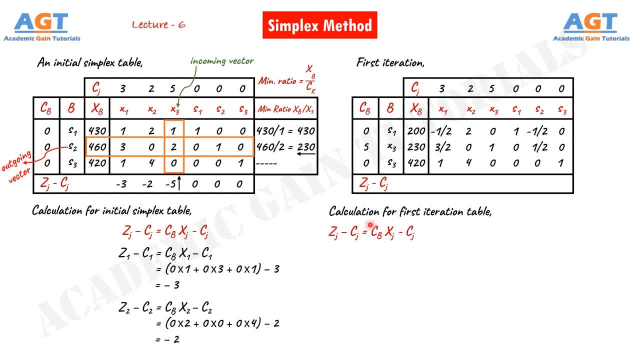 out the values for Zj minus Cj using this formula, just like we did for the initial table. The general formula is as follows. The formula is: Zj minus Cj equals to Cb into Xj minus Cj. 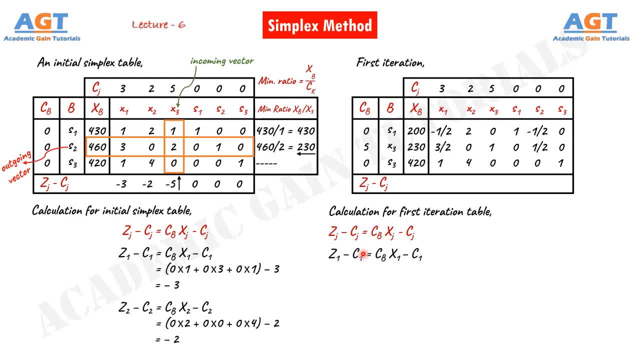 For the calculation of Z1, minus C1, the formula will be Z1, minus C1, equals to Cb into X1, minus C1.. In the initial table all the values of Cb were 0, but in this first iteration table 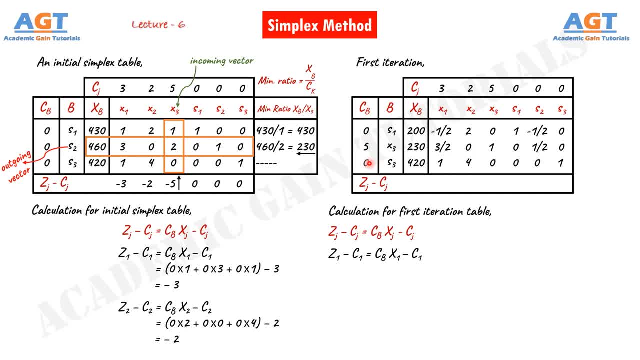 the values of Cb are 0,, 5, and 0. Here we have to multiply Cb with X1.. So 0 into minus 1 by 2, which gives us 0, plus 5 into 3, by 2, plus 0 into 1.. 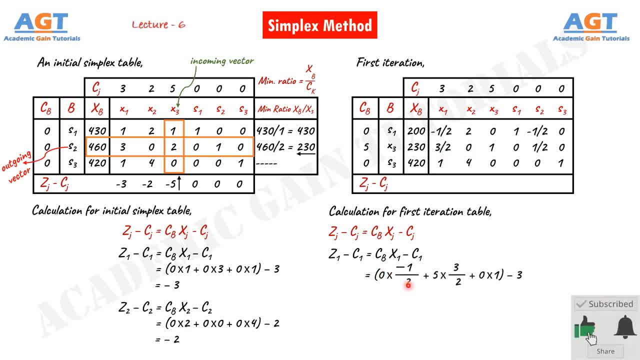 Now here we write: 0 into minus 1 by 2, plus 5 into 3 by 2, plus 0 into 1, then give the minus sign from formula and in the Cj row we can see the value of C1 is 3, so we write: 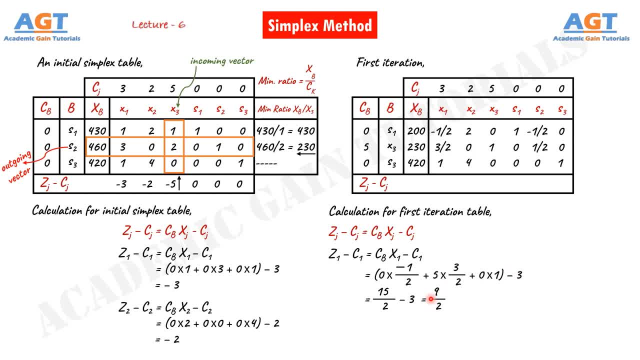 3 here. Similarly, the value of Z1 minus C1 will be 9 by 2.. So in this row here we will write 9 divided by 2.. Now in the same way, we will find out value of Z2, minus C2.. 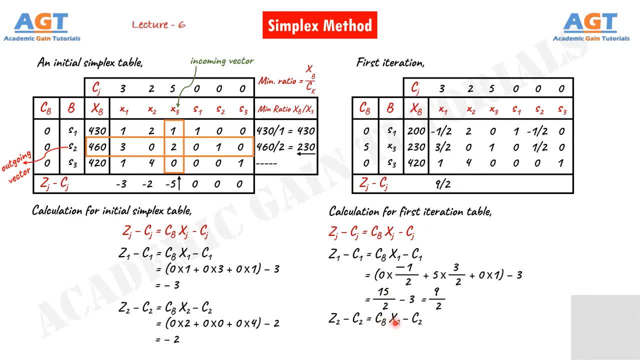 The formula will be Cb into X2, minus C2.. Here we will have 0 into 2, which gives us 0, plus 5 into 0, which gives us 0, plus 0 into 4, which gives us 0.. 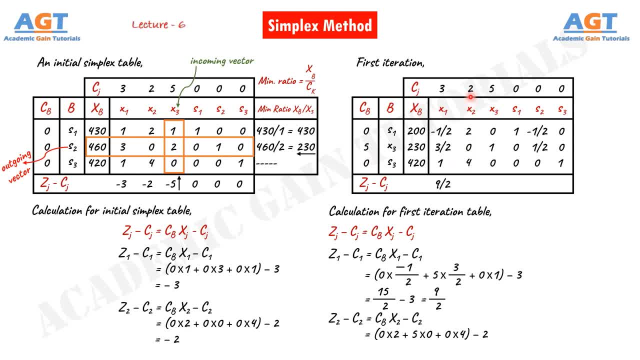 0.. So the value of cb into x2 will be 0, minus the value of c2 is 2.. And finally, the value of z2 minus c2 will be minus 2.. So in this row here we will write minus. 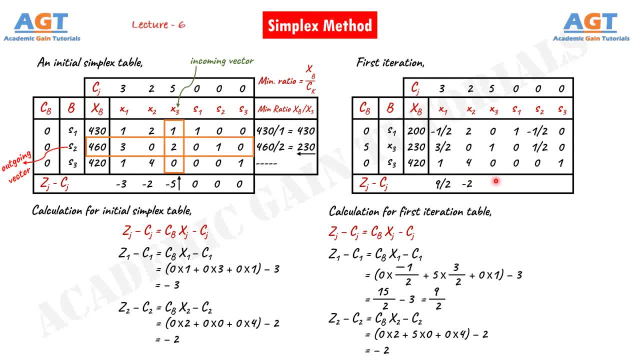 2. Now, in the same way, we will find out value of z3 minus c3. First multiply cb into x3. Here we will have 0 into 0, which gives us 0, plus 5 into 1,, which gives us 5, plus 0 into 0, which gives us 0. So the value. 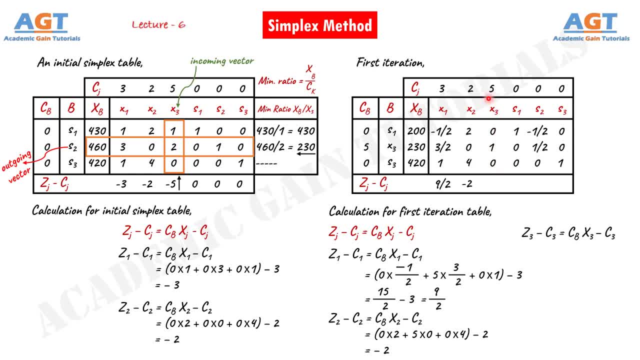 of cb into x3 will be 5, minus the value of c3 is 5.. And finally, the value of z3 minus c3 will be 5 minus 5, equals to 0. So in this row here we will write 0.. Similarly, 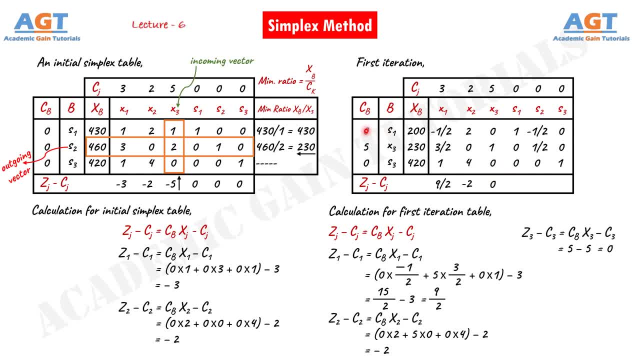 for z4 minus c4.. Here we will have 0 into 1, which gives us 0.. So in this row, here we will write 0.. For z5 minus c5, here we will have 0 into minus 1 by 2,, which gives. 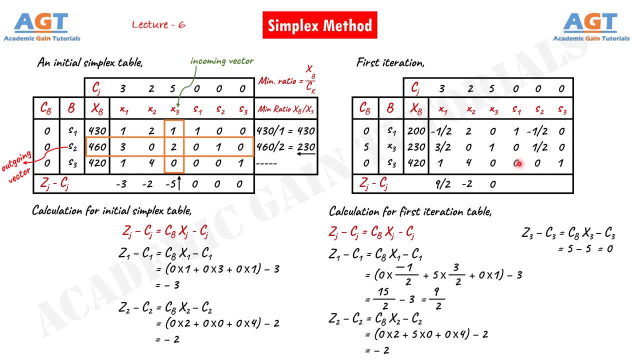 us 0, plus 5 into 0,, which gives us 0. So the value will be 0, minus the value of c4 is 0.. And finally, the value of z4 minus c4 will be 0.. So in this row, here we will. 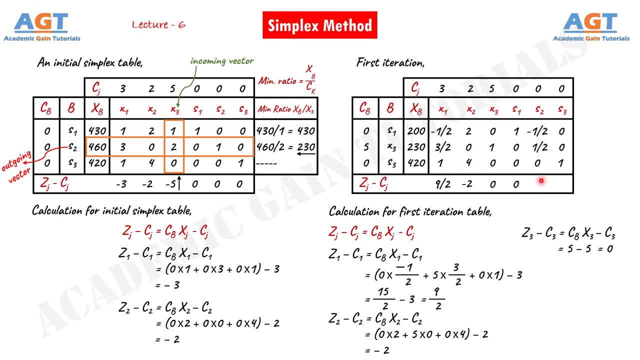 write 0.. For z5 minus c5, here we will have 0 into minus 1 by 2, which gives us 0, plus 5 into 1 by 2, which gives us 5 by 2, plus 0 into 0, which gives us 0.. So the value: 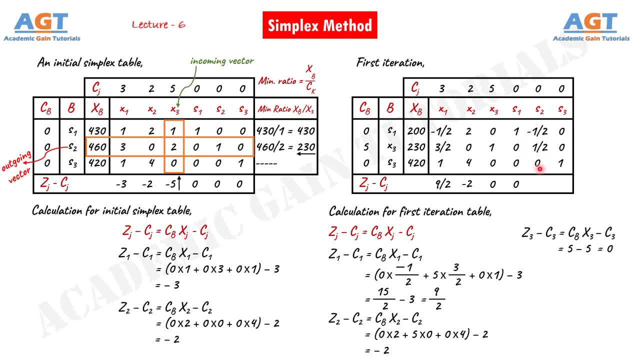 will be 5 by 2, as the other values are 0, minus the value of c5 is 0.. And finally, the value of z5 minus c5 will be 5 by 2.. So in this row here we will write 5 by 2.. And 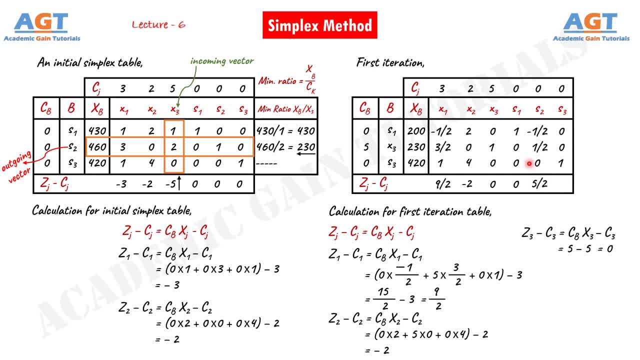 for z6 minus c6, here we will have 0 into 0,, which gives us 0.. So in this row, here we will write 5 by 2.. And for z6 minus c6, here we will have 0 into 0,, which gives. 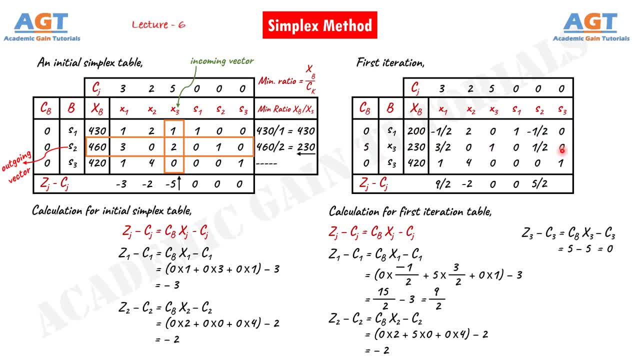 us 0.. So in this row, here we will write 5 by 2.. And for z6 minus c6, here we will have 0 into 0, which gives us 0, plus 5 into 0, which gives us 0, plus 0 into 1,. 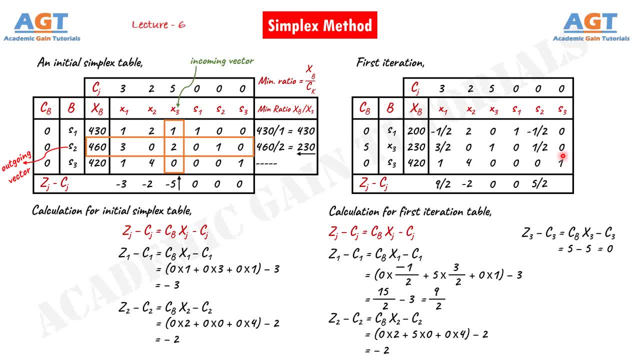 which gives us 0.. So the value will be 0, minus the value of c6 is 0.. And finally, the value of z6 minus c6 will be 0. So in this row here we will write 0.. Now we have. 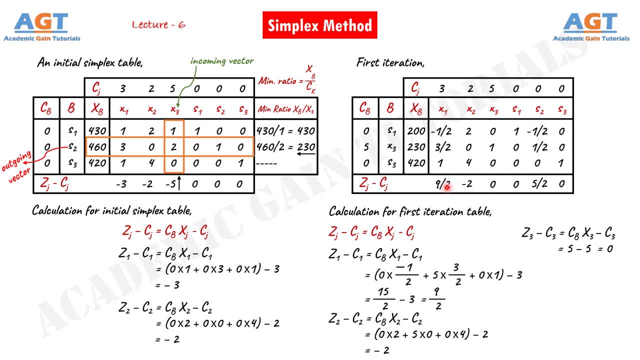 found out the values for zj minus cj and filled up this row. Here we can see a negative value of zj minus cj, which is minus 2.. We will indicate this negative value of minus 2 by an arrow And this column will be the key column. The variable x2 will be the incoming. 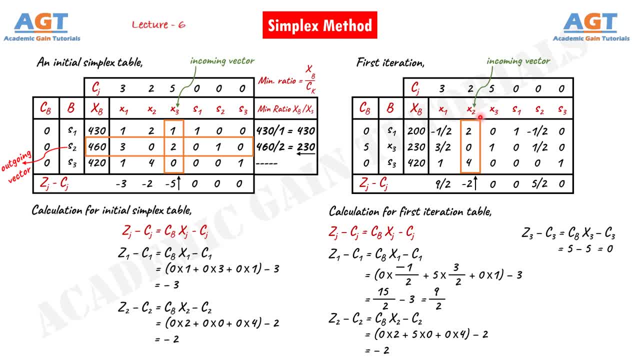 vector. Now, on this side, we will make a column for the calculation of minimum ratio. The formula for minimum ratio is xp divided by the key column, And the value of key column has to be greater than 0. Here the key column is x2.. So we will divide the values of column. 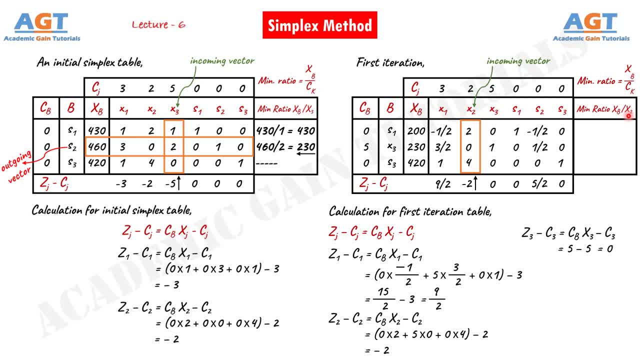 x2, by the values of key column x2 for calculating minimum ratio. For the first row, xp is 200, and value of x2 is 2.. So we divide 200 by 2, the minimum ratio will be 100.. For the 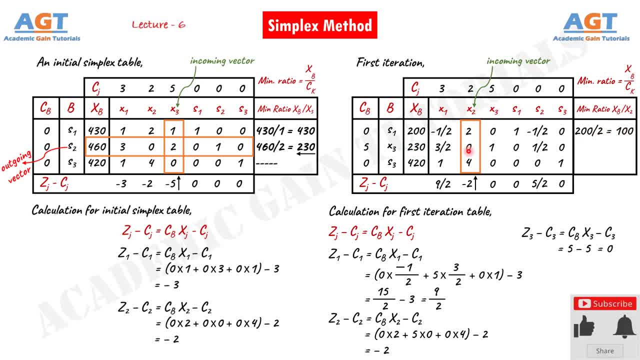 second row: xp is 230, and value of x2 is 0.. Since the value of the key column is 0 in this row, we will not calculate the minimum ratio for this row, because we said earlier that the value of key column has to be greater than 0,. it cannot be 0, or less than 0. Now 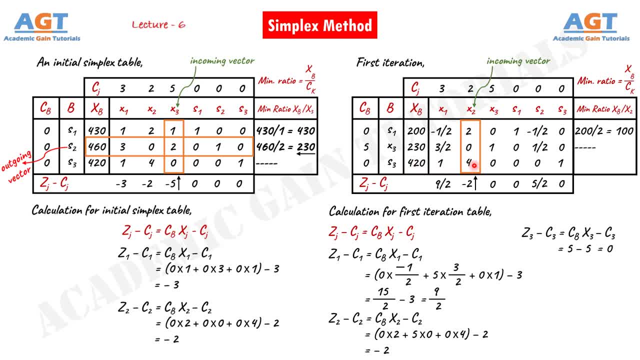 for the third row, xp is 420, and value of x2 is 4.. So we divide 420 by 4, the minimum ratio will be 105.. Now, between these two values, 105 and 100,, the minimum value is 100,. 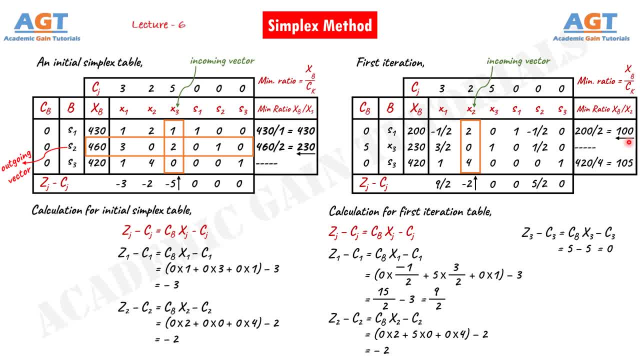 we will indicate this minimum value of 100 by an arrow and this column will be the key row. this variable s1 will be the outgoing vector And this common element between this key row and key column is called key element. Here, 2 is the common element between key. 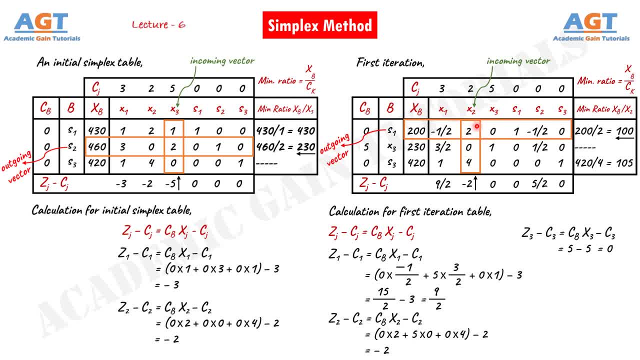 row and key column. so 2 is the key element. So in this first iteration simplex table, this is the key column. x2 is the incoming vector, this is the key row. s1 is the outgoing vector and this common element 2, is the key element. 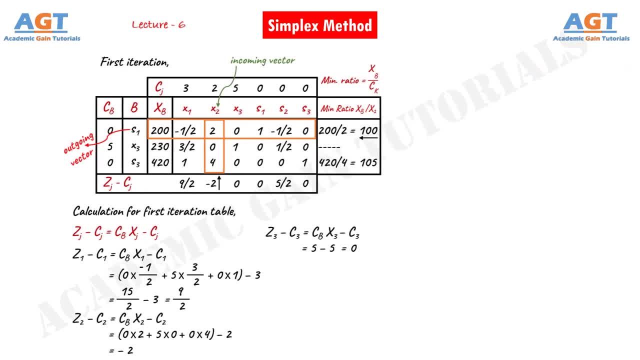 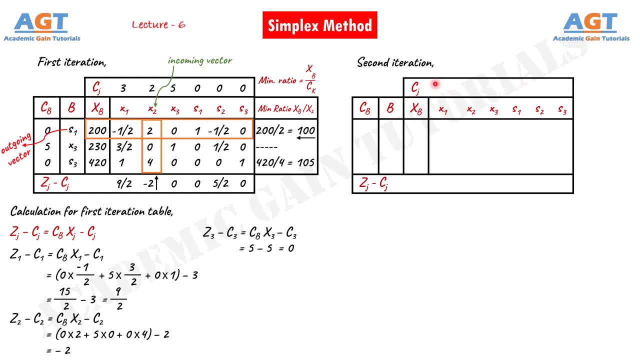 Now we will make the second iteration table. So here we have the simplex table for second iteration. The value of cj row will remain same because the cost of the objective function has remained same. So we will copy and write the value of cj from the first iteration table. 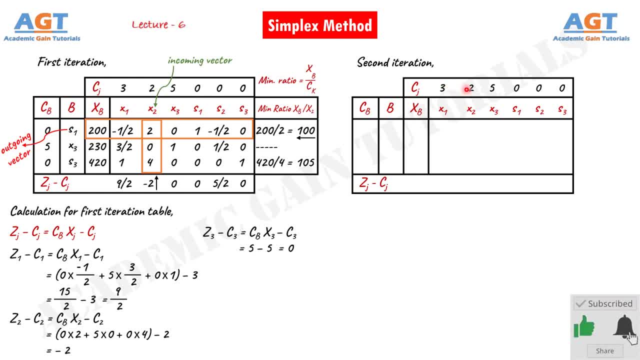 to this new table. Here we will write 3,, 2,, 5,, 0,, 0, and 0.. In the basic variable column in the first iteration table. In table we had S1, X3 and S3. 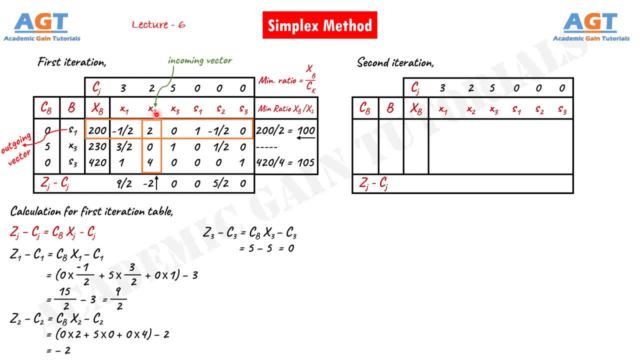 Here S1 is the outgoing vector, and in place of S1 the incoming vector is X2. So in place of S1 we will write X2.. Here we have written the basic variables X2, X3 and S3. So we have replaced S1 by X2.. 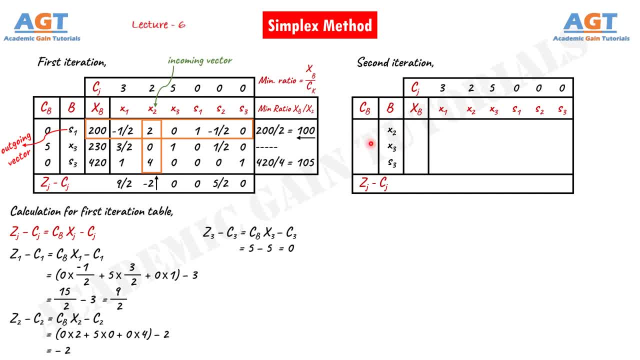 Now we will write the cost of these variables here. So the cost of X2 is 2, the cost of X3 is 5 and the cost of S3 is 0.. Now we have to fill up the rest of this table by doing the calculations. 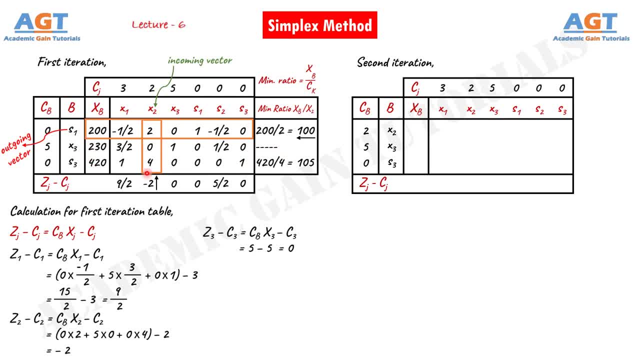 In the first iteration table we saw one method of finding the values. In the first method we cross, multiplied the old values to get new values. Now, in this second iteration table, we will see another method of calculating the values to fill up the table. In this second method we will find out the values. 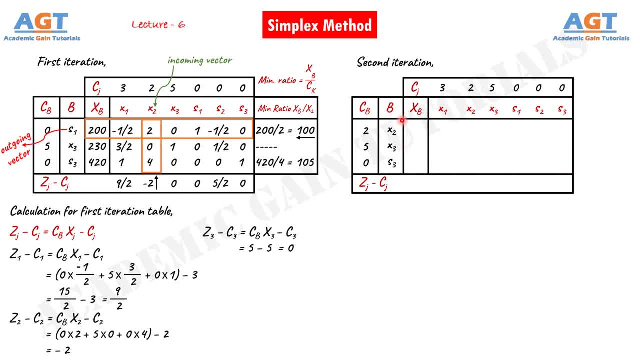 By doing some row operations and column operations. you can either use the first method or this second method that we will see now, whichever seems easier to you. So for the first row, we will divide all the values of the key row by the key element. 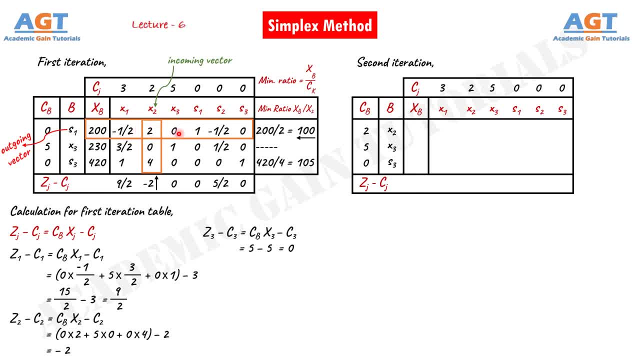 So we divide 200 by the key element 2, which gives us 100.. Divide minus 1 over 2 by the key element 2, which gives us minus 1 by 4.. Then divide key element 2 by 2. This gives us 1.. 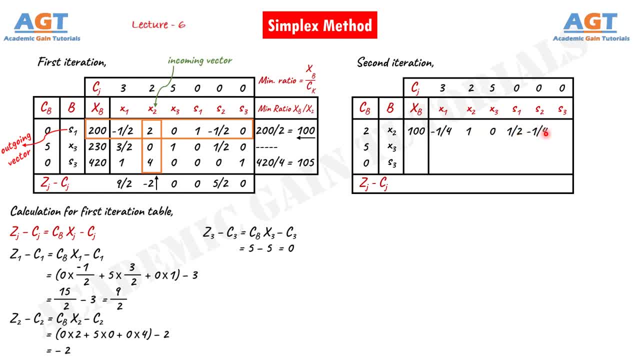 Here we will have 0, then 1 by 2, minus 1 by 4, and 0.. So why did we divide this whole row by 2? Since this is the key row. here we have the key element. 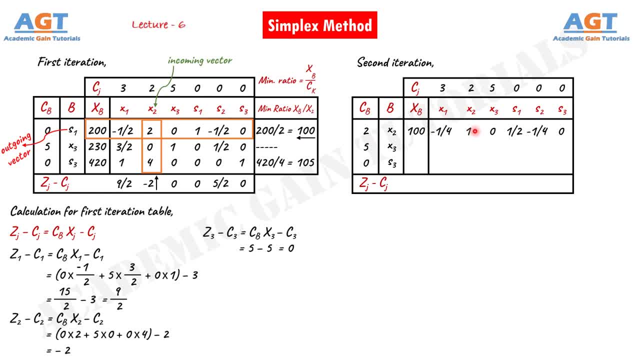 When we make the new table, the key element has to be changed and written as 1.. Now if we divide the key element 2 by 2, then in the second iteration table we will get 1 in the same position Again, since we cannot divide just one element from the row. 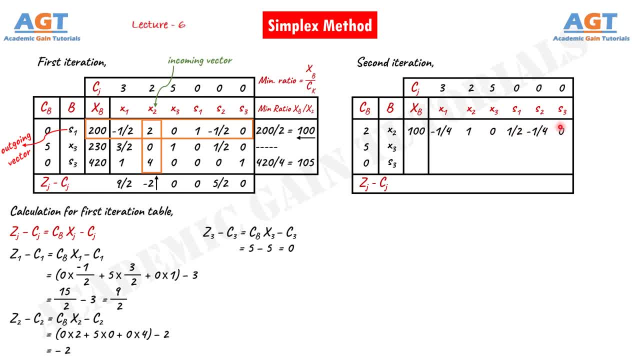 We divided the whole key row by 2 and got this new row in the second iteration table. As we can see here, the key element 2 has been converted into 1 in this new table. So we have shown the key element of this key column as 1 in this new table. 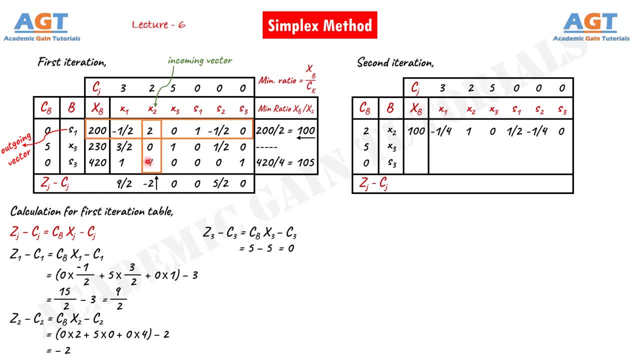 Now we have to show the other two elements of the key column as 0.. Now this second value of the key column is already 0, so we don't have to change anything in this row to make it 0.. We will write this row in the new table as 1.. 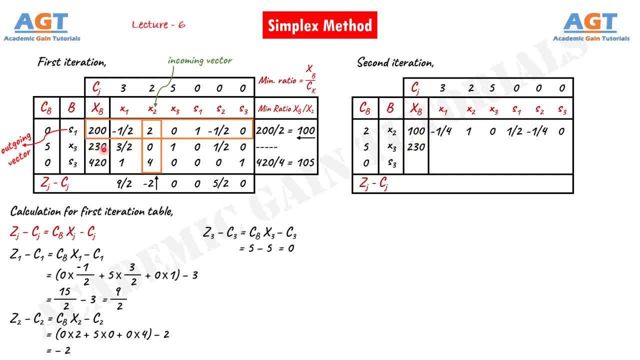 So here we write 230,, 3 by 2,, 0,, 1,, 0,, 1 by 2, and 0. So the first element of the key column has been converted to 1.. The next element is 0.. 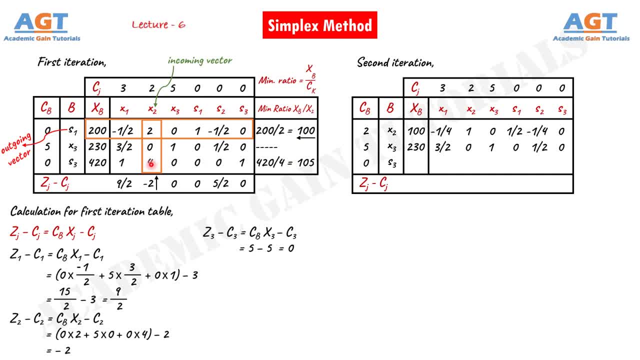 Now the third element of the key column is 4.. We have to do some row operation to convert 4 to 0 in this new table. So the row operation for this third row will be: r3 dash equals to i3 dash, Now r1 minus 4r1.. 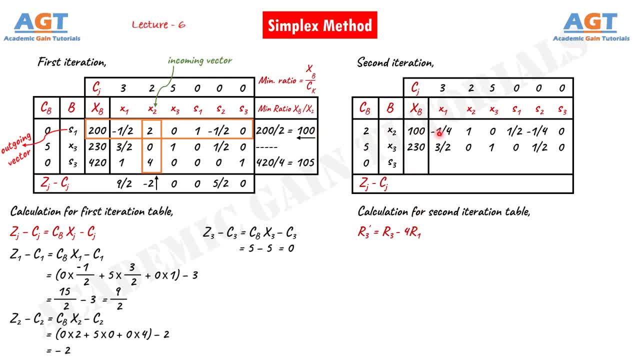 We will use r1 to solve this operation, Because r1 was the key row in the previous table. we have to get 0 in the position of 4 here. so in this row operation we will multiply this new first row by 4 and then subtract. 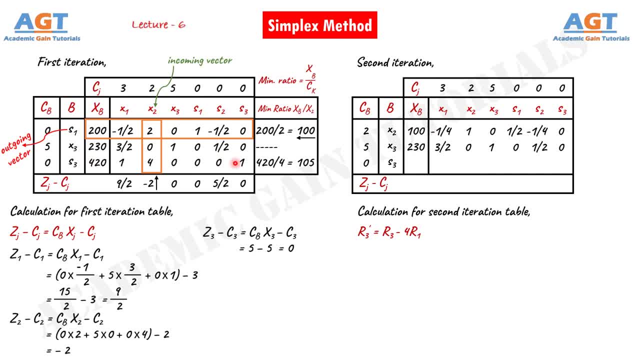 from the old column's third row. Let's see in rough To get the new row 3, r3 dash. first we will write the old row 3.. 420.. 1, 4, 0, 1, 3.. 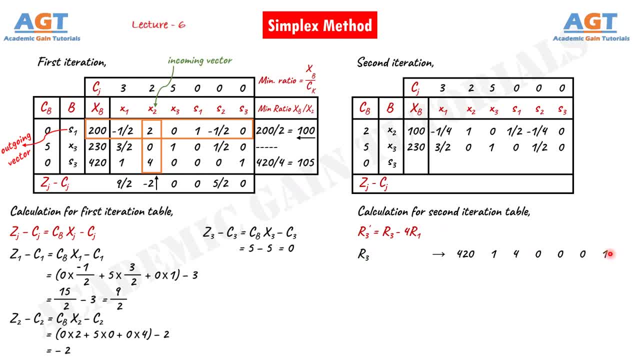 Then r1, and then 4.. 1,, 4,, 1,, 2,, 3.. 0,, 0, and 1.. So this is our 3.. Then we multiply this new row 1, by 4, and right here so. 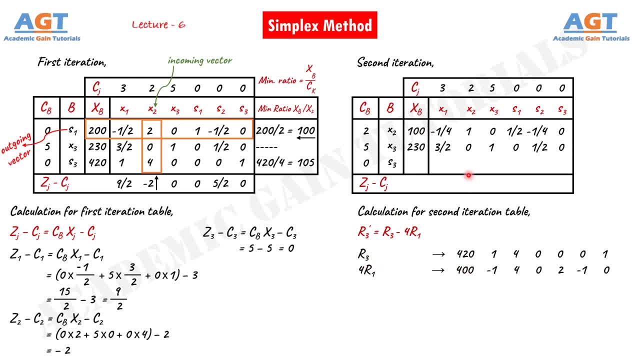 4 into 100, gives us 400,. 4 into minus 1 by 4, gives us minus 1.. Then we have 4, 0,, 2, minus 1, and 0. So this is 4r1.. Now subtract 4r1, from our 3,, we get 20,. 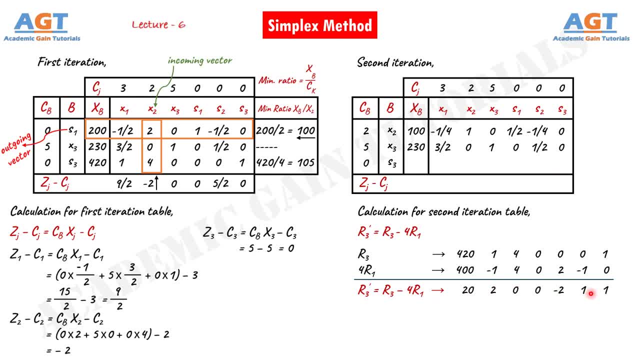 2, 0, 0, minus 2, 1, and 1.. So this is our 3 dash, or the new, our 3 row. Now we will put this: values of new, our 3 row: 20, 2, 0, 0, minus 2, 1, and 1.. Now, if we look carefully, 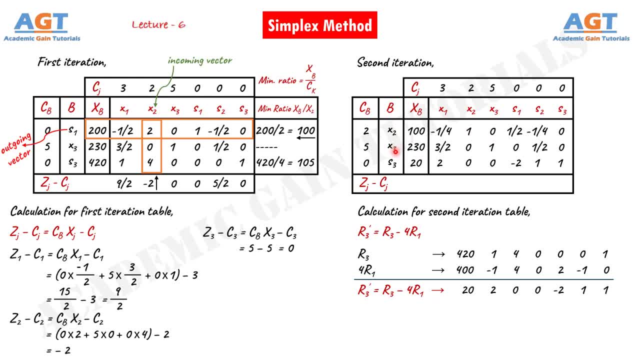 in this table the basic variables are x2, x3, and s3.. If the x2, x3, and s3 columns are arranged in the same serial, we should get an identity matrix, as we have seen earlier Here. the first basic variable: 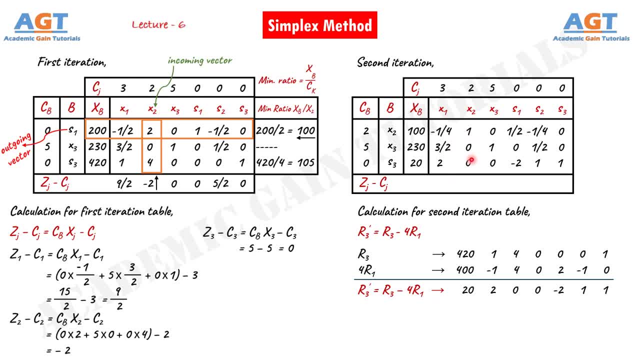 is x2, in the x2 column we have 1, 0, 0.. Now the second basic variable is x3, in the x3 column we have 0, 1, 0.. And the third basic variable is s3, in the s3 column we have 0,. 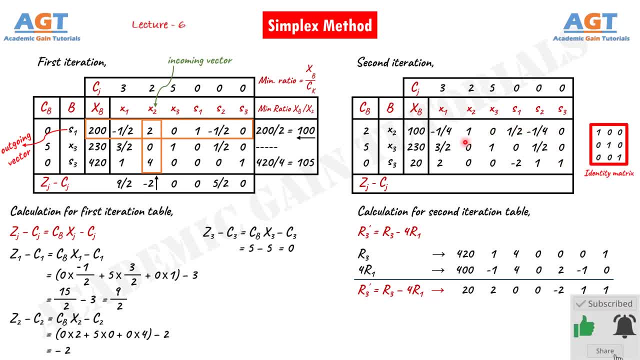 0, 1.. Now if we arrange the columns of x2,, x3, and s3 serially, we will get an identity matrix form like this one. Now we will find the values for the zj minus cj row. We have seen how to calculate zj minus cj in the previous. 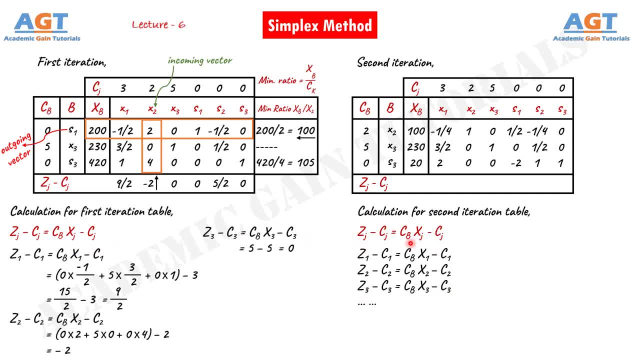 two tables, so let's calculate them quickly. For the calculation of z1, minus c1, here we have to multiply cb with x1.. So 2 into minus 1 by 4, plus 5 into 3 by 2, plus 0. 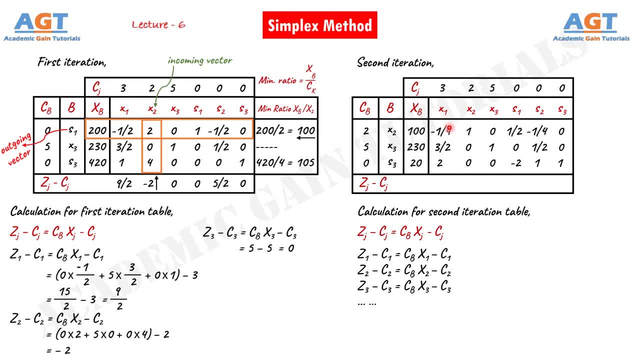 into 2.. Now we have to solve it And in the cj row we can see the value of c1 is 3, so we will subtract 3 from the value of cb into x1. And finally, the value of z1 minus c1 will be. 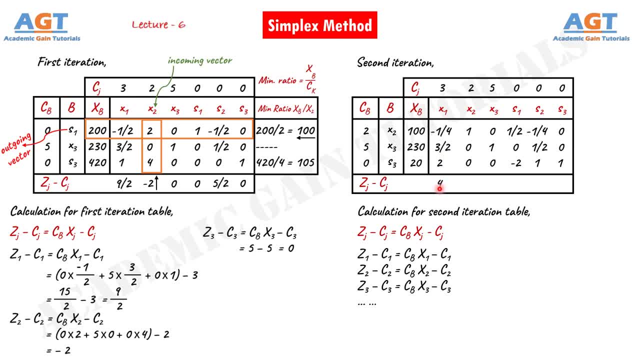 4,. so in this row here we will write 4.. Now, in the same way, we will find out value of z2, minus c2.. First we have to multiply cb with x2, so 2 into 1, plus 5 into 0,. 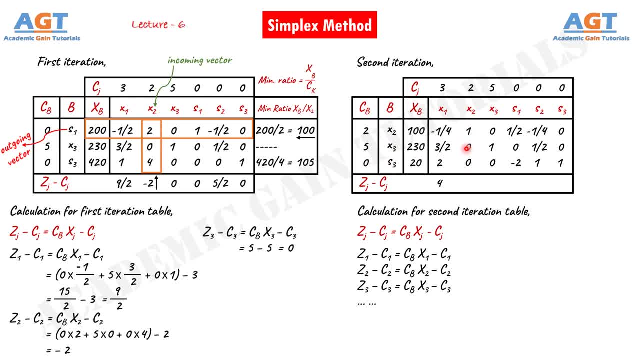 plus 0.. Then we will solve it And in the cj row we can see the value of c2 is 2.. So we will subtract 2 from the value of cb into x2.. And finally the value of z2 minus c2 will be. 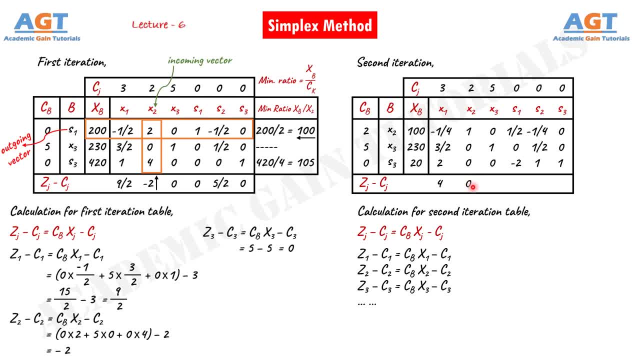 0.. So in this row here we will write 0.. If you want, you can write the detailed calculation in rough and check the values, Since we have seen the detailed calculations for zj minus cj in the previous tables. we. 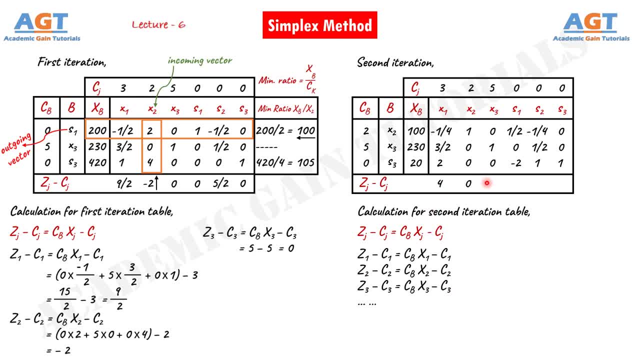 are solving quickly now. So in the same way we will find out value of z3 minus c3.. First multiply cb into x3. Here we will have 2 into 0, plus 5 into 1, plus 0 into 0. So the value of cb into. 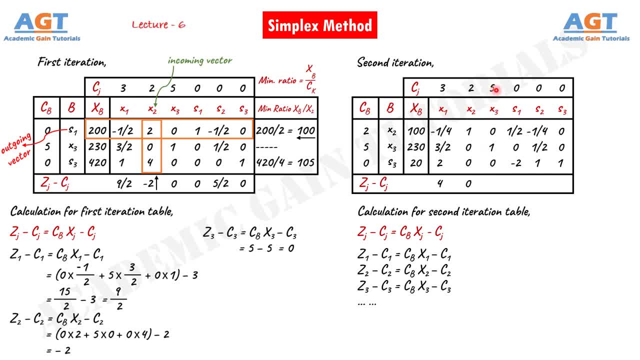 x3 will be 5, minus the value of c3 is 5.. And finally, the value of z3 minus c3 will be 5 minus 5, equals to 0. So the value of c3 minus c3 will be 5.. And finally, the value of z3 minus c3 will be. 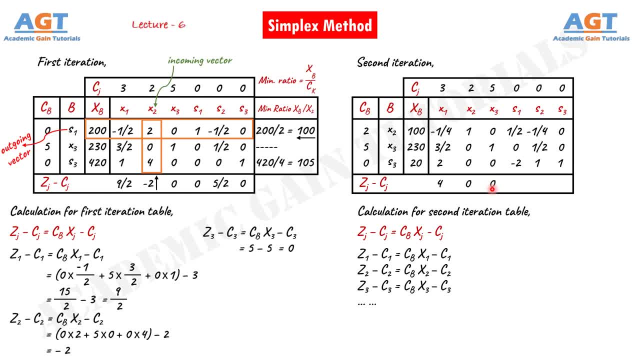 In this row, here we will write 0.. Similarly for z4 minus c4, here we will have 2 into 1 by 2,, which gives us 1, plus 5, into 0, which gives us 0, plus 0 into minus 2, which gives us 0.. 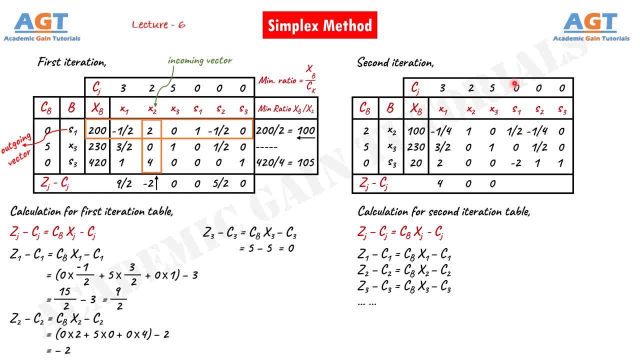 So the value will be 1, minus the value of c4 is 0, and finally, the value of z4 minus c4 will be 1.. So in this row here we will write 1.. 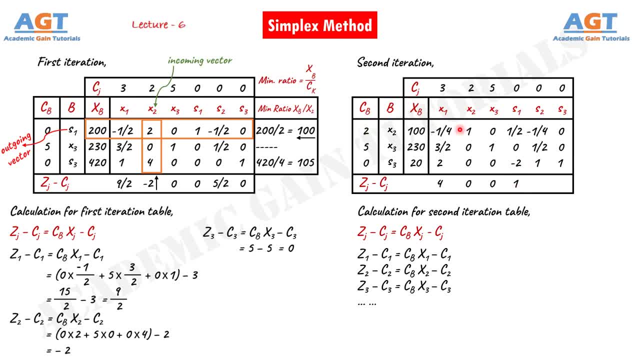 For z5 minus c5, here we will have 2 into minus 1 by 4, plus 5 into 1 by 2, plus 0 into 1, minus, the value of c5 is 0, and finally, the value of z5 minus c5 will be. 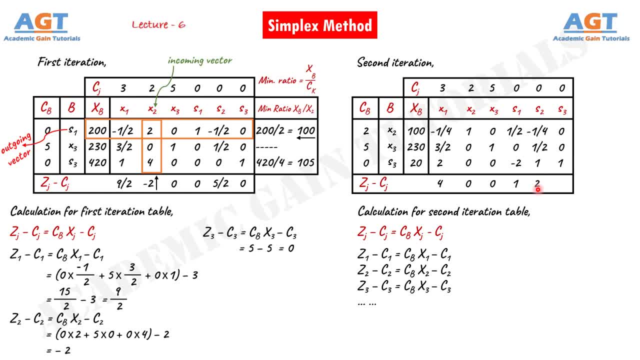 2.. So in this row, here we will write 2.. And for z6 minus c6.. Here we will have 2 into 0, plus 5 into 0, plus 0 into 1, minus the value of c6. 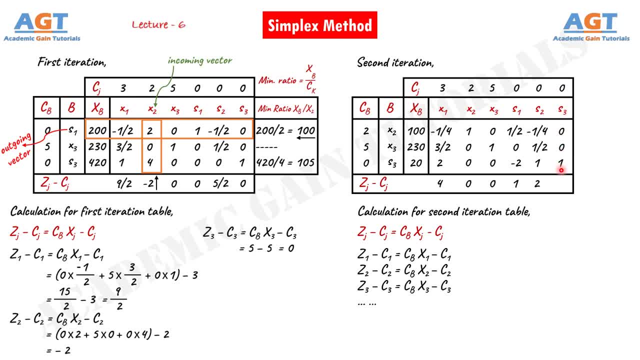 is 0, and finally, the value of z6 minus c6 will be 0.. So in this row here we will write 0.. So we have found out the values for zj minus cj and filled up this row. 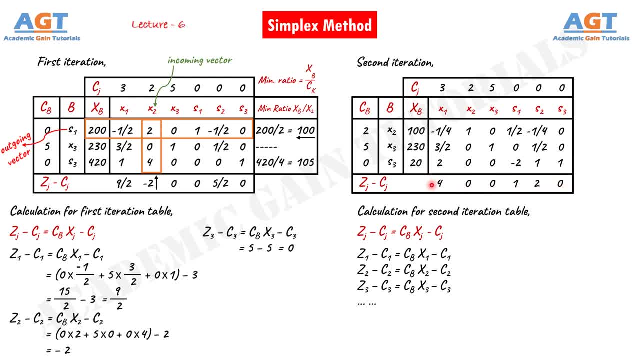 Now, if we look at the values of zj minus cj, all these values are either greater than 0, or equal to 0, there is no negative value of zj minus cj here, since all the values of zj minus cj are greater than or equal to 0, that is, they are all positive values. 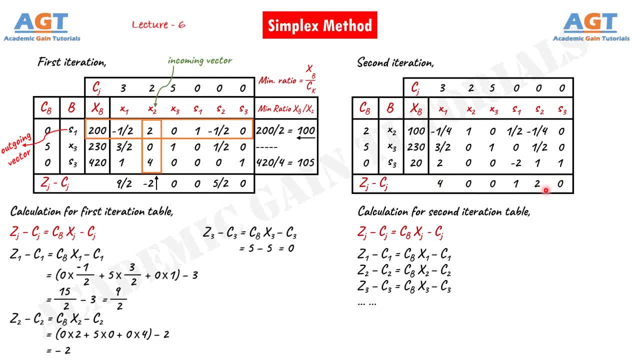 So we can say that our solution has reached the optimal stage. Finally, we will write: since all values of zj minus cj are greater than or equal to 0,, the solution is optimum. Then we will write the values of x1,, x2, and x3. 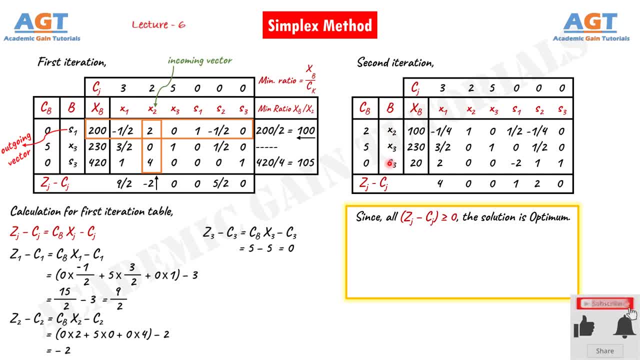 So we have all the values of zj minus cj. So we have all the values of zj minus cj And x3. from the basic variables Here we can see that value of x2 is 100, value of x3 is 230, and there is no x1. 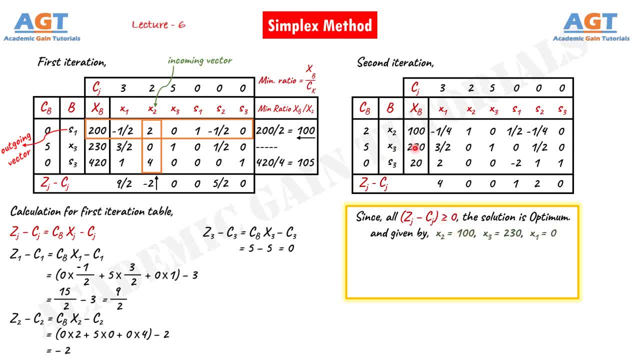 So we write: x2 equals to 100,, x3 equals to 230, and x1 equals to 0. Now in our objective function we had maximize z, So we will calculate max z here. The formula of max z will be: 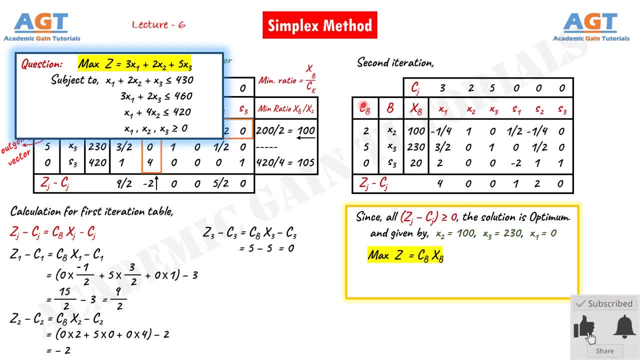 cb into xp. Now we will multiply values of cb with xp and then we will add them In cb column. here we have 2,, 5, and 0, and in the xp column we have 100,, 230, and 20.. 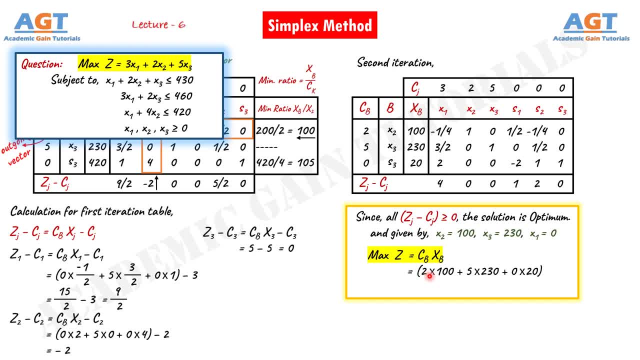 So we will write cb into xp equals to 2 into 100, plus 5 into 230, plus 0 into 20.. The answer will be 1350.. So we will write cb into xp: equals to 2 into 100, plus 5 into 230, plus 0 into. 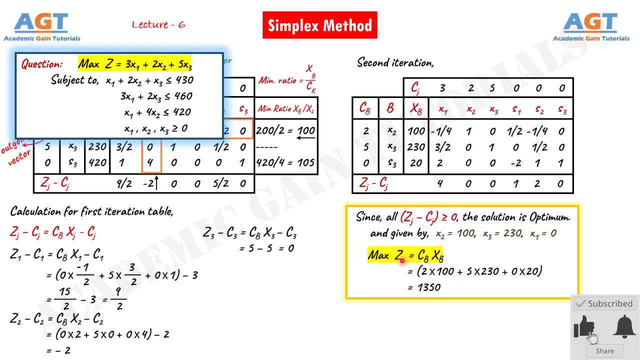 250. Thus the optimum value of max z is 1350.. So in this lecture we have solved a maximization problem by simplex method. In the next lecture we will solve a minimization problem by simplex method. Thank you for watching this video. if this video was helpful, give it a thumbs up. subscribe.